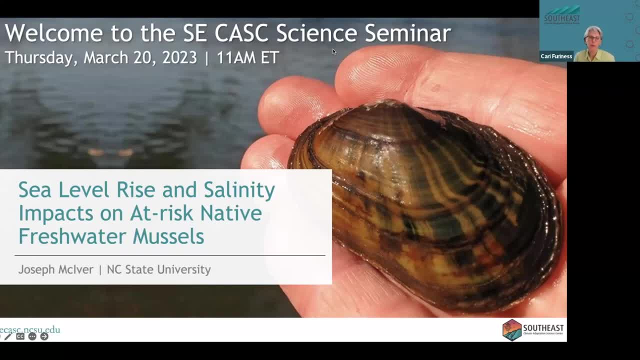 Let me start by letting you know what to expect from today's webinar. We'll go over some quick meeting logistics And then request some feedback, And then request some feedback from those of you who've joined via a quick poll, And then I'll introduce our speaker for today. He'll present for 40 to 45 minutes or so and then we'll have time for Q&A and discussion at the end. before we wrap up. 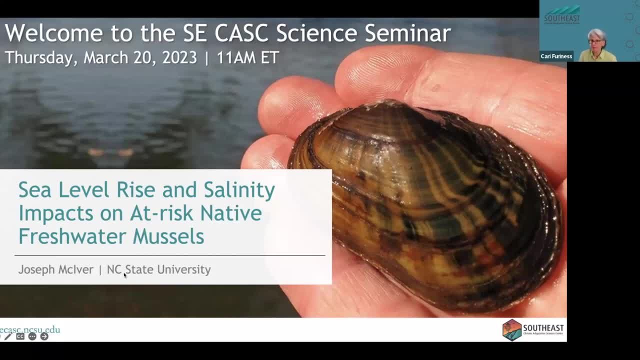 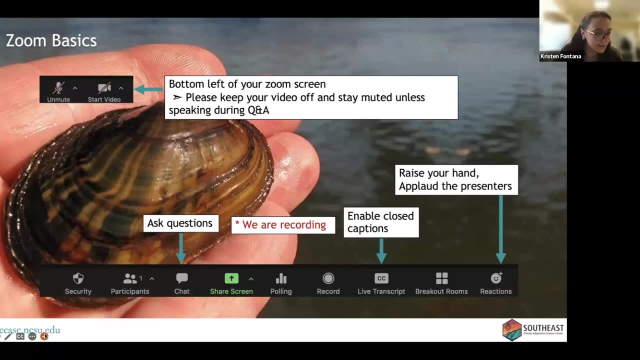 So now Kristen will give you a quick overview of our webinar technology. Hi, I'm just, yeah, going to quickly cover some Zoom features that we're using in this webinar. I'm sure that we're all pretty familiar with Zoom at this point. 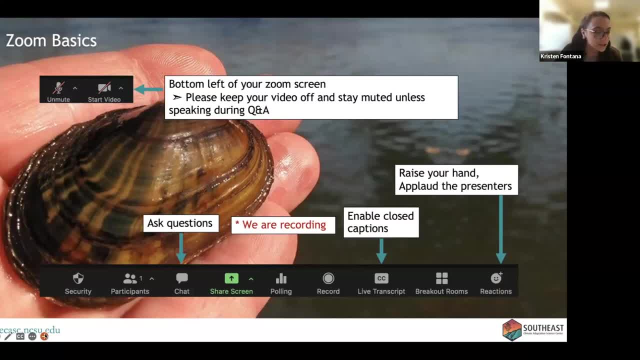 But we do recognize the context. Some folks do use different technologies, So I'll just point out a few things for you guys. The controls on the bottom left of your Zoom screen allow you to mute and unmute yourself. We will keep all lines muted and ask that you also keep your video off so that we can reduce distractions during the presentation. 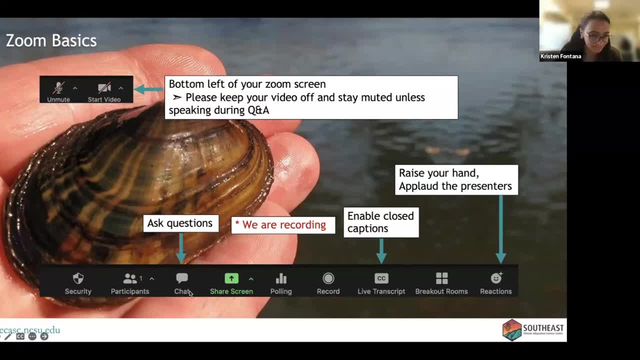 In the middle of the bottom bar you can access the chat window And I encourage you, if you have questions during the presentation, to submit them in the chat for discussion after the talk. We'll be monitoring the questions there And we'll pose them to our speaker during the Q&A session. 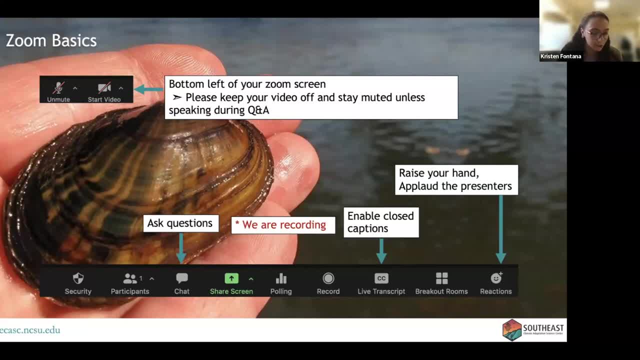 We will also be recording today's webinar And you can access and share the recording afterwards on the Southeast CASC website, on our Science Seminars webpage and on our YouTube channel. Now we're going to launch a short poll just to get a bit of information about who is with us and to help us know how to continue to get information out about these seminars. 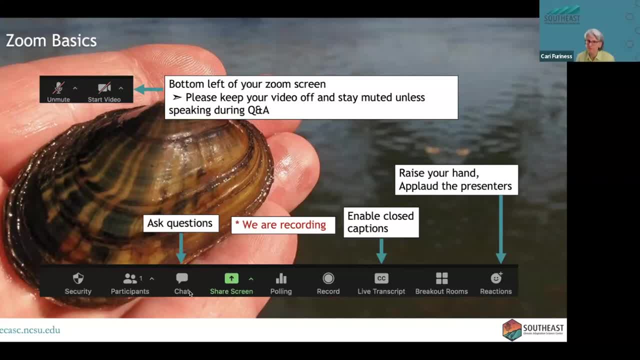 So we'll give you about half a minute or so to fill it out, So I'll share the results here. Thank you everyone for filling it out. Thank you everyone for filling this out and for feeding back this information. 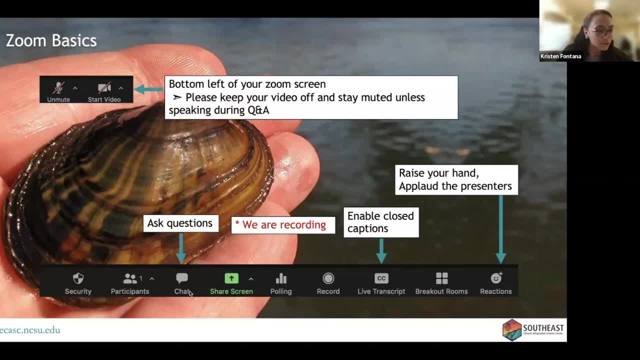 It's great to see the breadth of folks in our audience today, which sets us up for a robust discussion about this research. Now we'll turn over to our presentation. While we switch screen sharing, Carrie will introduce our speaker. Yeah, great. 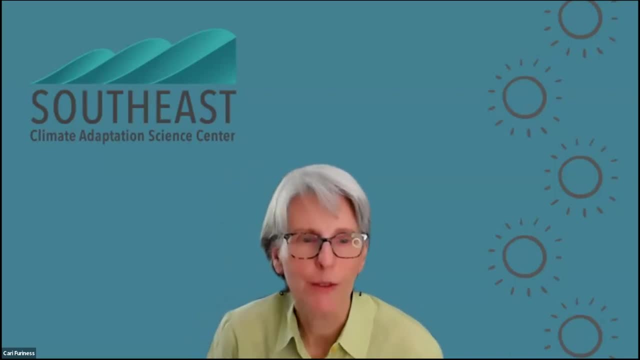 Yeah, and thanks y'all for reading our newsletter, which is obviously where some of you got this information, So I appreciate that. So, yeah, so I am delighted, Joseph, if you want to start to get your screen share up. 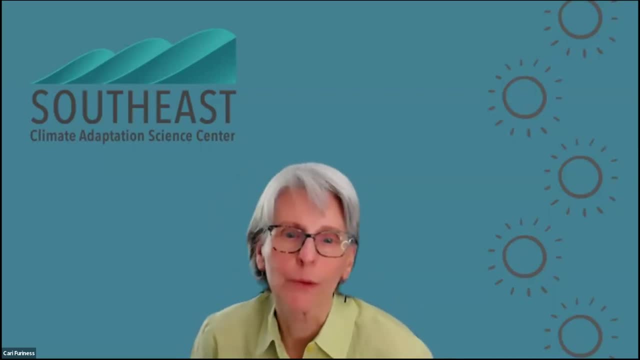 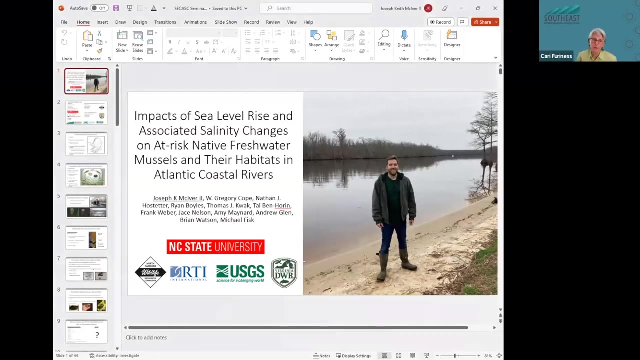 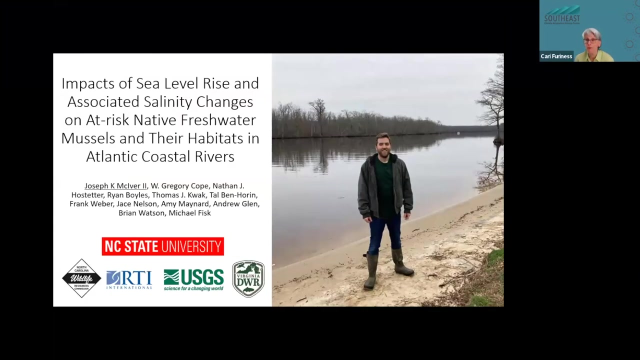 I'm delighted to introduce our speaker today, Joseph MacGyver. So Joseph is a recent graduate of North Carolina State University, where he investigated the impact of sea salt on freshwater mussel viability in organ systems as part of a CCASC-funded project, and his Master of Science degree 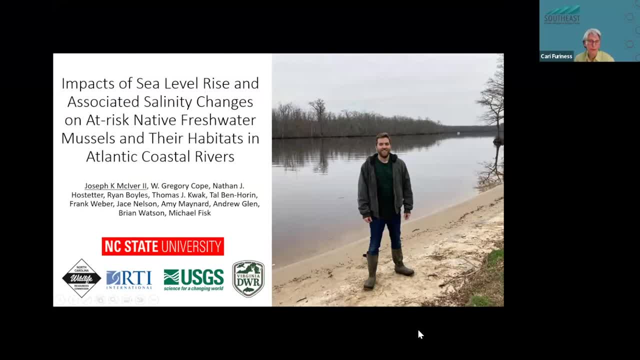 So Joseph has held a variety of environmental positions in the private sector with the state of North Carolina and academia since 2015.. And he was recently awarded the Richard L Noble Best Student Presentation Award By the North Carolina Chapter of American Fisheries Society when presenting these research results. 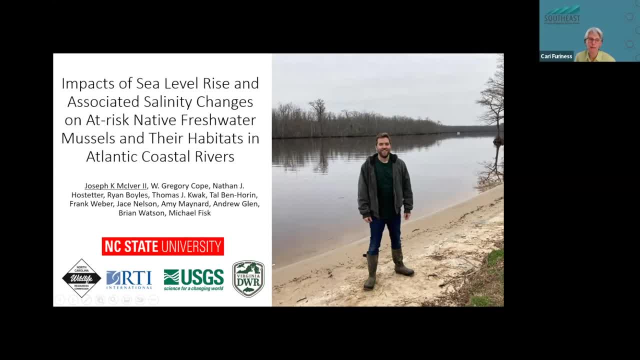 So the title of his presentation today, you can see, is impacts of sea level rise and associated salinity changes on at-risk native freshwater mussels and their habitats in the Atlantic, in Atlantic coastal rivers. So now I'll turn it over to you, Joseph. 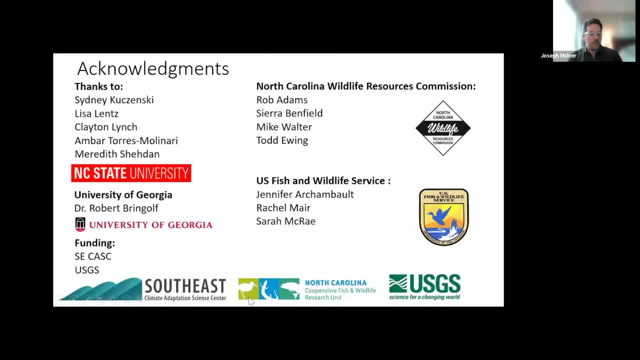 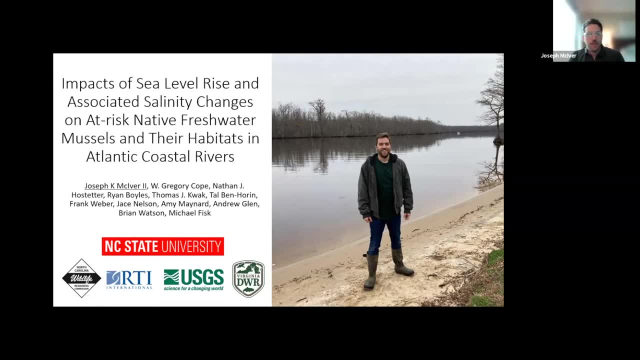 Thanks, Carrie, for the introduction. Oh, already having some challenges, Okay, Well, as she stated, I'm here to talk about my research I've recently wrapped up focused on the challenges with salinity changes in these coastal river systems due to sea level rise. 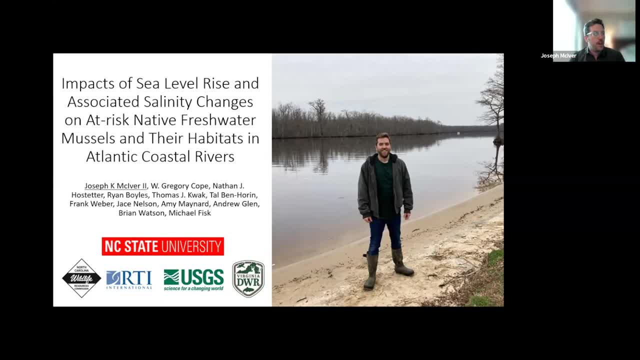 So first I'd like to thank my co-authors I have listed here. They helped me a ton and they did a lot of good work, and I appreciate all of them very much. I'd like to go ahead and acknowledge everyone else who helped me here, including. 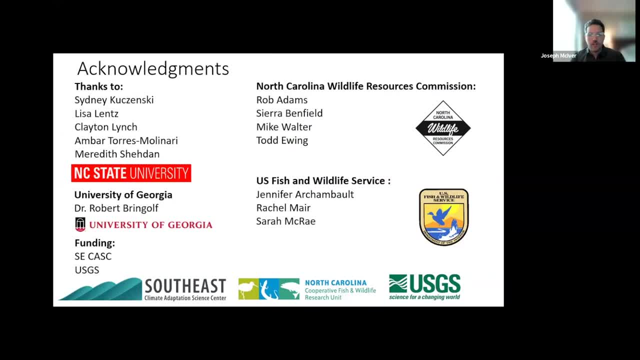 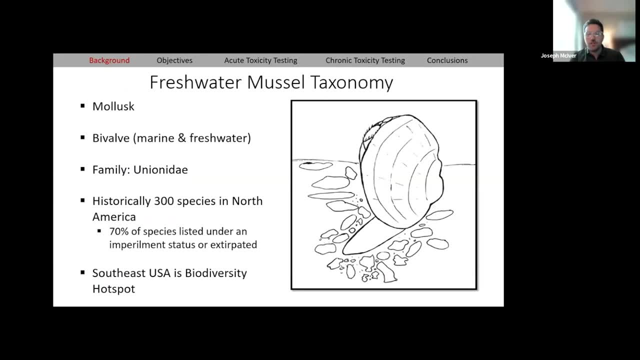 Our funding sources, which is USGS, and our host, the Southeast Climate Adaptation Science Center. So first let's get into this. We're going to get a little background on freshwater mussels and the ecology and salts and then we'll get into the meat of this research. So I'm glad to have you all here. So freshwater mussels, they are a mollusk, they're a bivalve, two halves of a shell. 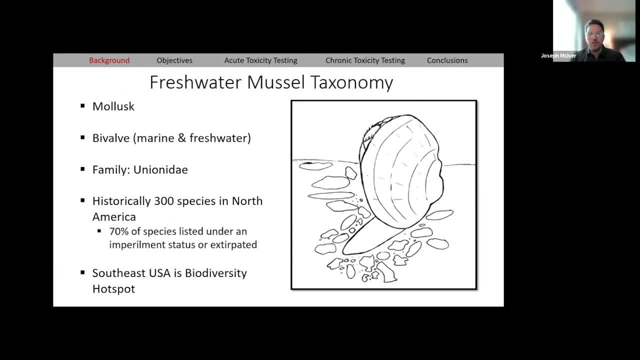 These were specifically focused on the family unionidae. Historically, there were 300 species in North America and 70% of those are listed under some sort of imperilment status In the Southeast United States of America is the biodiversity hotspot for these animals in the world, So this is the place to be for freshwater mussels. Southeast United States. 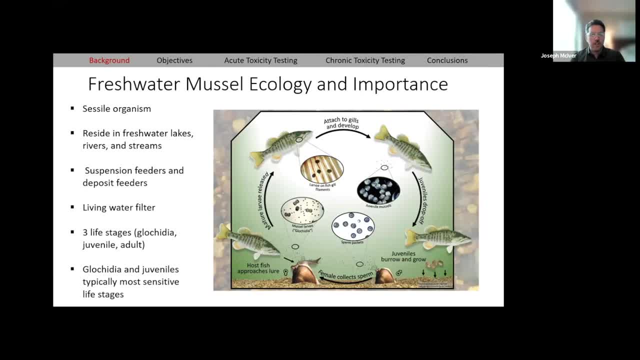 A little bit about their ecology. They're a sessile organism. They essentially they don't move really. They can move vertically up and down In the substrate, so in the bottom of a stream or a river they reside in, like I said, streams or rivers or lakes. 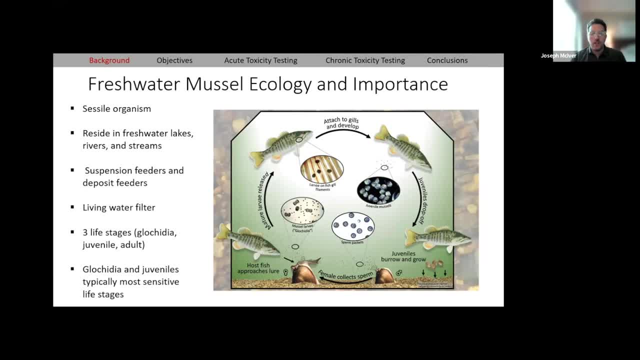 They feed on suspended particles in the water and they also can feed on particles within the substrate they're living in. There's three life stages, So the glochidia- which, if you can see the cursor here, the glochidia are these little tiny ones, They're the larval stage, The juveniles, which are right here, and the adults. 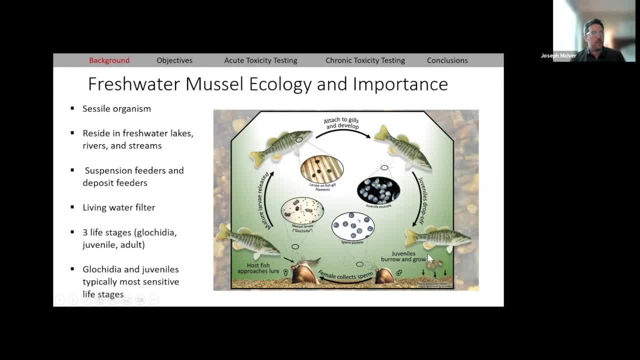 So the adults are the ones that are producing these babies And they have a really unique life cycle where- which I've depicted here or have put up this slide here- where they require a host fish for their reproduction, So they lure in a host fish with this little lure here. 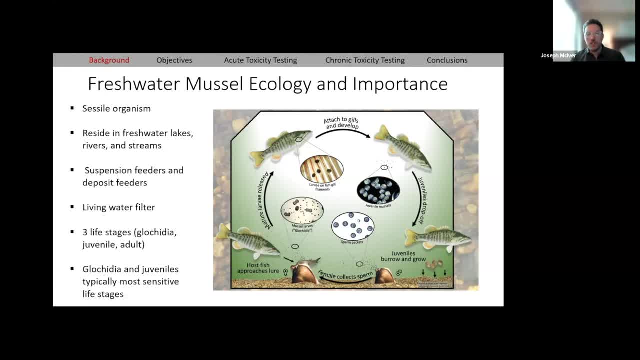 The fish will clamp on, thinking it's a prey item, that will release the glochidia, which will then attach right here on their gills or even fins, where they will develop into these juvenile muscles, And then they'll drop off into the sediment where they can grow. 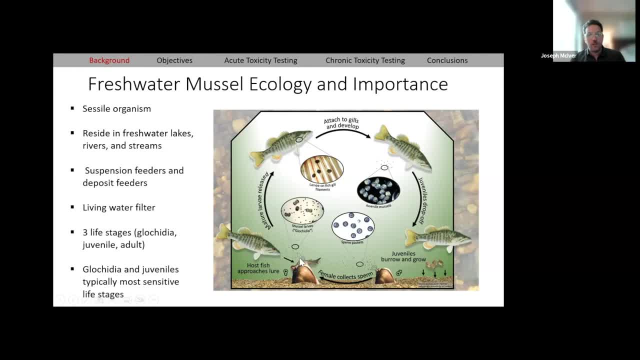 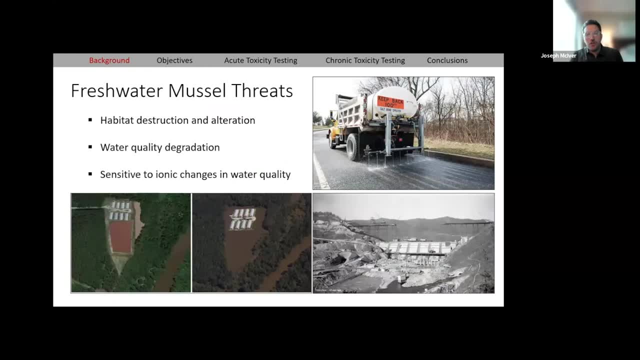 And typically the glochidia life stage. so these really little, tiny, tiny babies are the most sensitive life stage to different challenges. So that brings me to kind of some of these challenges or threats to freshwater mussels. The big ones are habitat destruction, alteration, water quality degradation, and they're really sensitive to ionic changes in water quality. 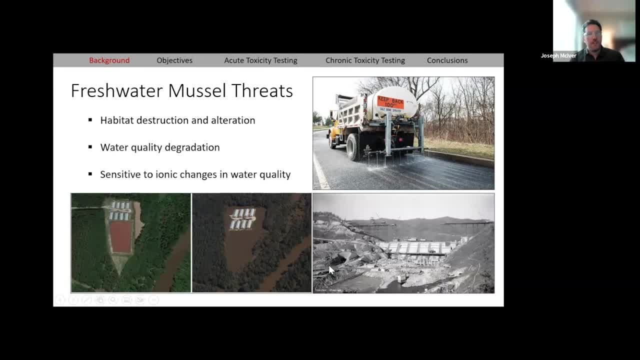 So I think these photos do a pretty good job of displaying those challenges. The bottom right here is a photo of Fontana Dam in North Carolina getting built, So it's impacting that river system- an increase of sediments that has to do with the construction of the dam. 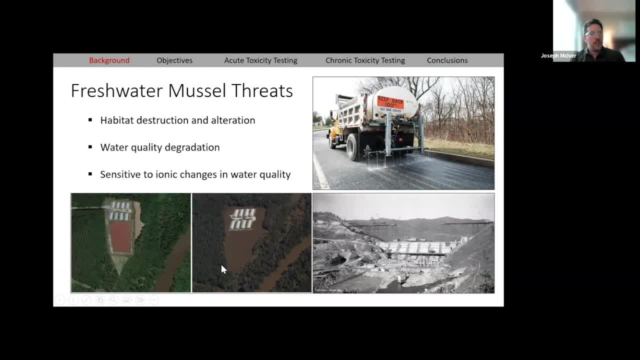 These two photos here on the left, this is a hog farm in North Carolina that was flooded in 2016 due to Hurricane Matthew. So this kind of reddish Brown color that's the sewage lagoon of this hog farm. So it was flooded and all of that sewage and all of those, you know, whatever is in there, all that nastiness ended up getting into the river system, which is right there. 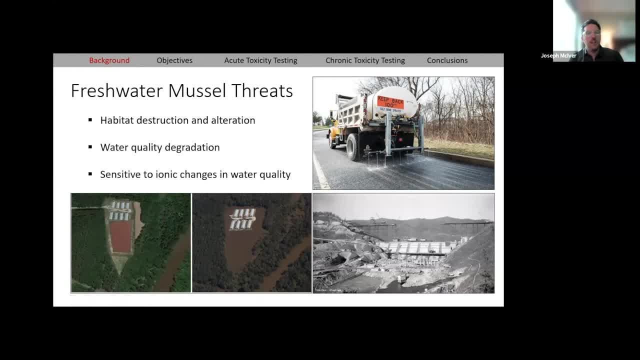 So that's an example of how some toxicants can get into there. But what I wanted to focus on with this talk is salt, so the salinity. So this right here is a brine truck putting down a solution in preparation for a snow or ice storm, you know, to keep the snow or ice from sticking. 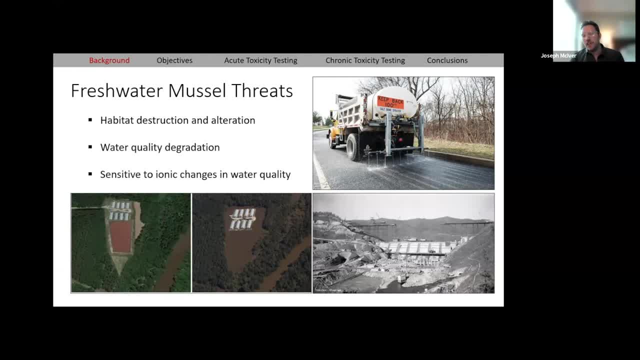 But once that thaws out, once the storm's over and it gets warm and the ice is gone, those salts end up getting into the river system, which is not too terribly good for freshwater mussels. So that brings me to focusing on the salts. 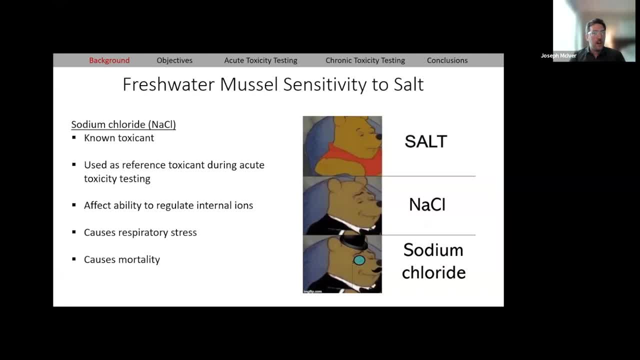 So right now I just want to talk about sodium chloride In ACL. it's a known toxicant to freshwater mussels. It's used as a reference toxicant during acute toxicity tests. You can affect their ability to regulate their internal ions and it can cause respiratory stress, so it can mess with their gills. 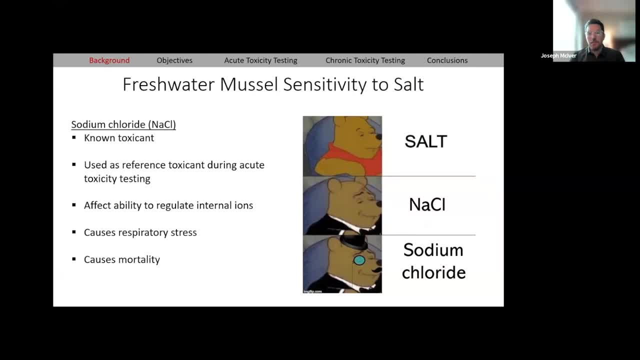 It can cause mortality to these animals. And this is Winnie the Pooh. I just thought this was a nice little picture of Winnie the Pooh getting a little educated on salt. So now I want to give some background on what an acute toxicity test is. 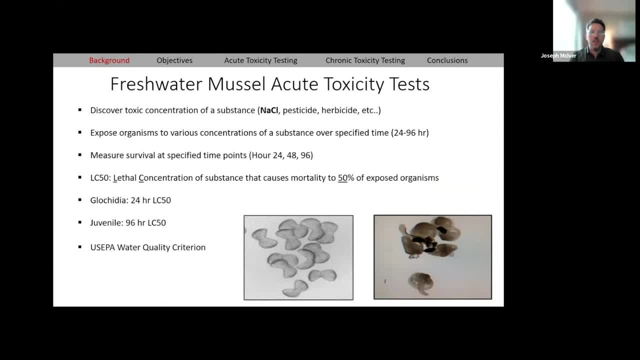 So typically acute toxicity tests are done to discover the toxic concentration of a substance, For instance sodium chloride. So you expose your organisms, in this case your freshwater mussels, to various concentrations of that substance over a specified time. 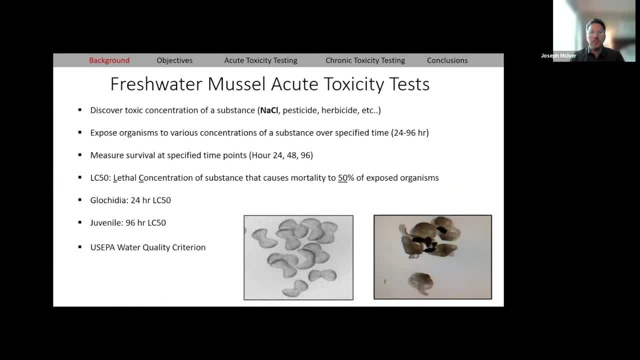 For freshwater mussel acute toxicity tests. those typically last from 24 to 96 hours, depending on what life stage you're looking at here, And then you'll measure the survival of those animals at specified time points. So this is the total of the total of those animals: 24,, 48, and 96, of the test. 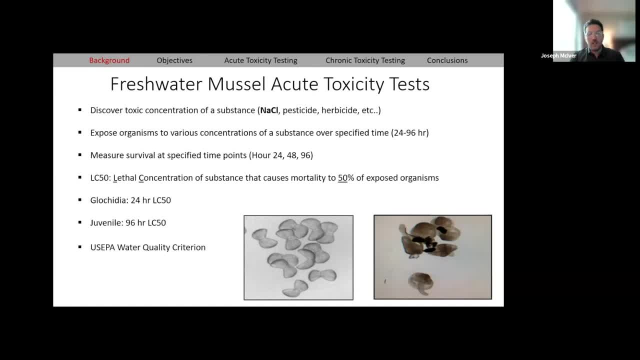 And what you're looking for mainly is you want to find the LC50, so the lethal concentration of that substance that causes mortality to 50% of those exposed organisms, or mussels And for glochidia you're really focused on this 24-hour LC50.. 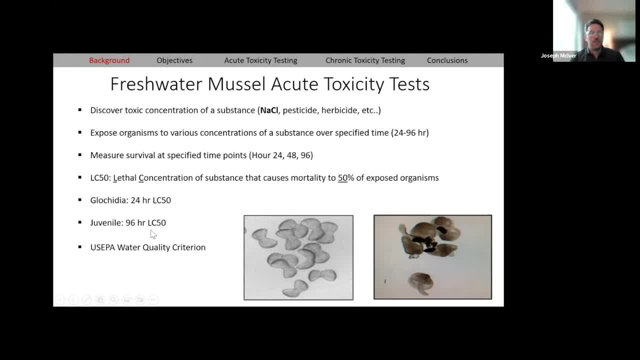 And for juveniles, you are focused on the 96-hour LC50, because those are the two time points that the US EPA uses to see whether or not a human is at risk of death. And for juveniles, you are focused on the 96-hour LC50, because those are the two time points that the US EPA uses to see if someone has diabetes. 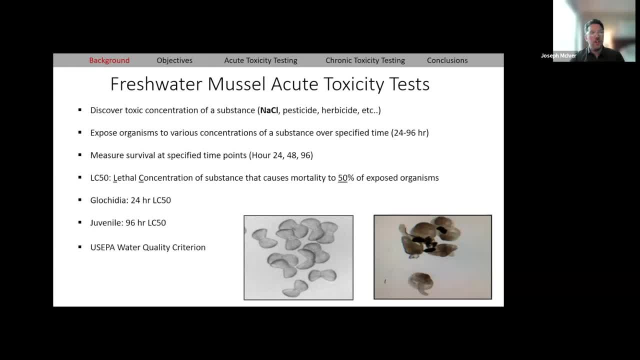 And for women, it's important that they're at risk of death, And for women, it's important that they're at risk of death- set their water quality criteria. And so those are the big ones right there. Next, I want to give. 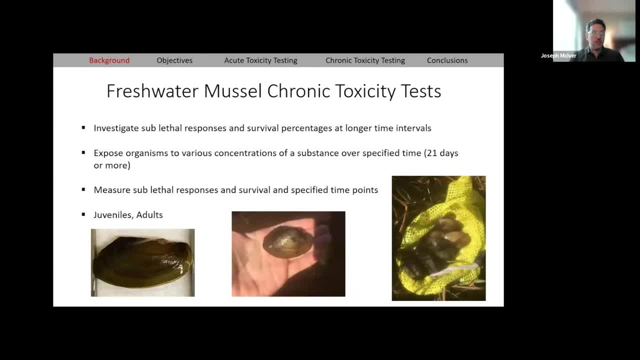 some background about chronic toxicity tests, So this is a little different than acute. This is more looking at sublethal responses and sometimes survival percentages of older freshwater mussels- So sub-adults, juveniles- and it's looking at these over longer time periods. So the minimum. 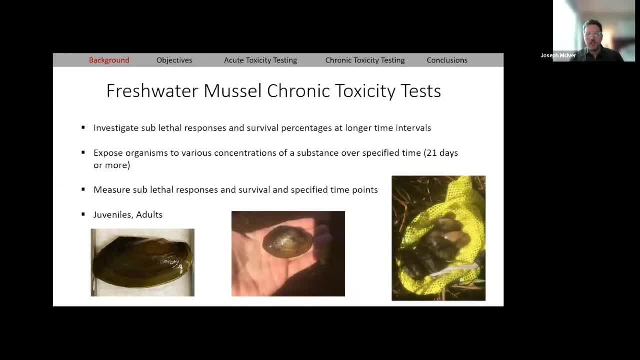 time period for a chronic toxicity test is 21 days. Some of them last for months and months. So chronic is a little flexible, but minimum is 20, 21 days And again you're exposing them to a toxicant and measuring those sublethal or survival, those responses at your specified 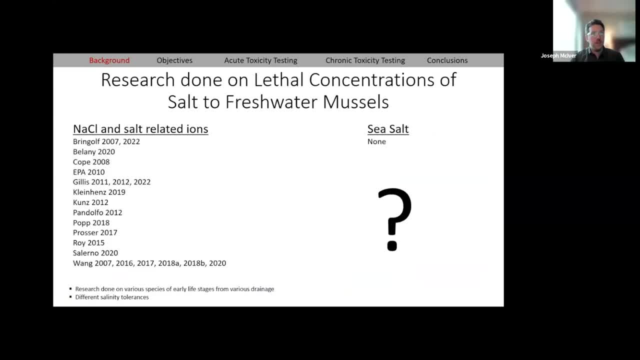 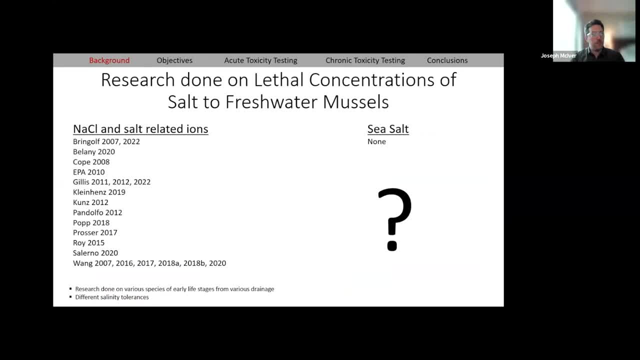 those are the lethal concentrations, So those LC50s of salt to freshwater mussels. There's been a fair amount of research done with sodium chloride and salt-related ions, But I'm here to talk about sea salt And to my knowledge there has not been any research done on the 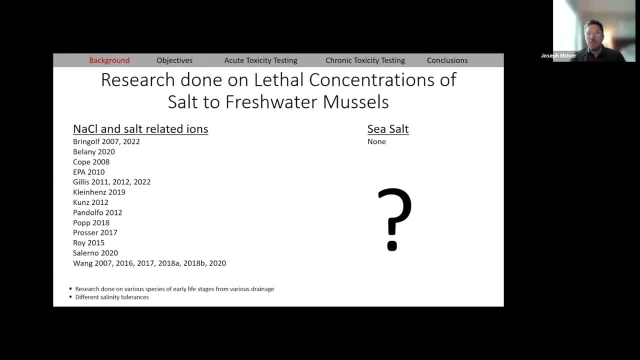 lethal concentrations. So finding those LC50s of sea salt to freshwater mussels, So that's kind of a knowledge gap that we thought was needed and that we could fill. So that's what we're doing at sea salt And that's why we started to look at salt. But why are we looking at sea salt? 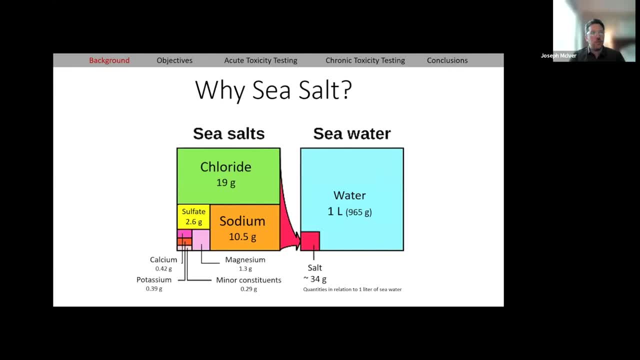 These are freshwater animals. What's the difference between sodium chloride and sea salt? So this picture, I think, does a pretty good job of explaining that. This is showing the amount of salt in a liter of seawater. So that box on the right is a liter of seawater And then it kind of 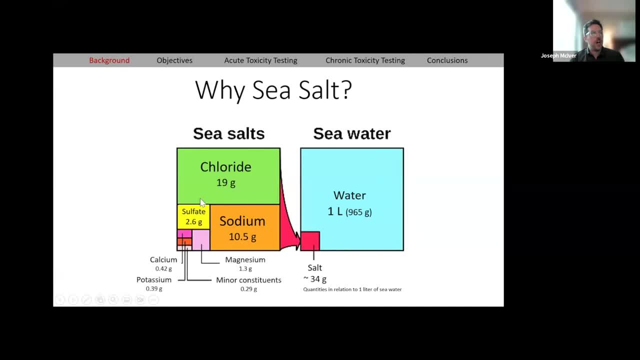 juts out and says: okay, this is the concentration of each ion within that salt solution, enk, And in a third we get more and more salt in the shore, And then over a few years we've been getting more and content. so it's predominantly sodium chloride, but also contains these other constituents here, like 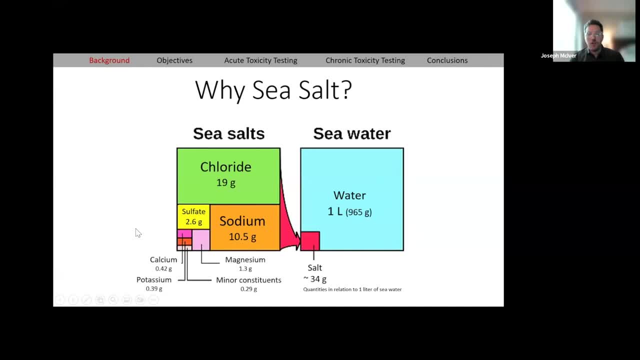 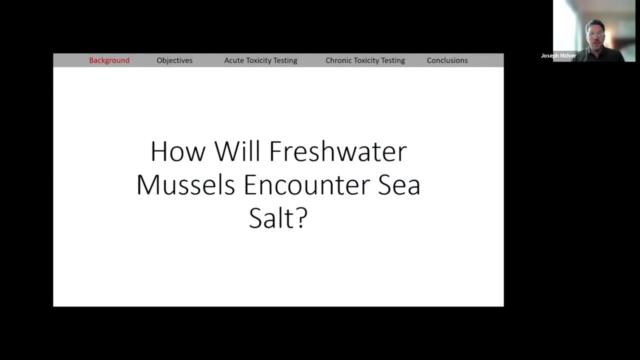 sulfate and calcium and potassium. so that hasn't really been looked at before- this kind of mixed toxicity effect of sea salt to freshwater mussels. but these live in fresh water. how are they going to encounter this sea salt? the idea and the cause could be climate induced sea level rise. 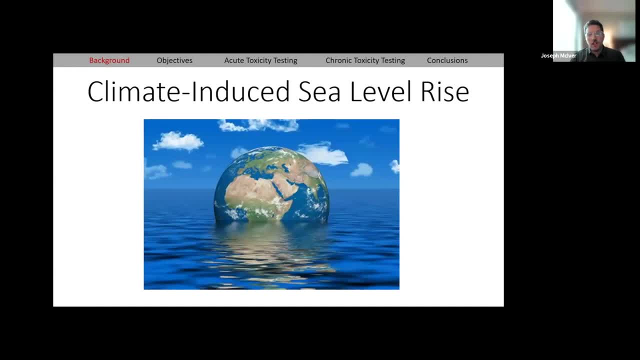 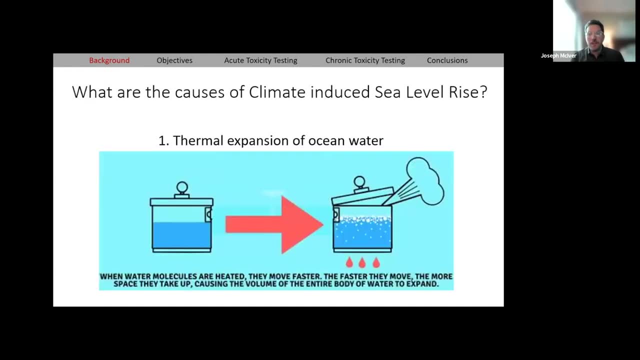 so what is that? what you know, it's kind of self-exploring explanatory sea levels coming up and getting into these freshwater habitats. but how is this sea level rise happening? what are the causes? so, number one, one of the main causes. there's really two main causes, and number one, the thermal expansion of ocean water. so that's kind of 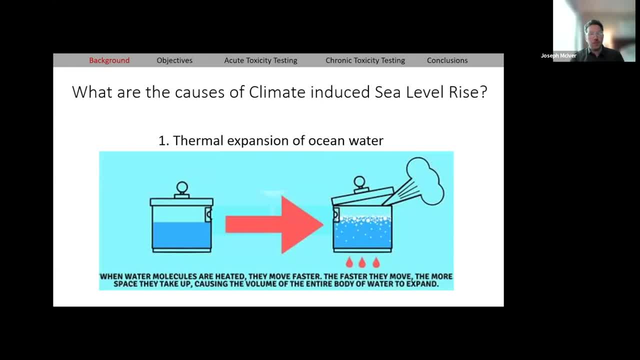 as water heats up, it expands and it needs somewhere to go, kind of like this, this pot boiling over. if you've ever done that, that's the same principle here. um, your water is getting hot and it's got to go somewhere and it's going to go up and into rivers. 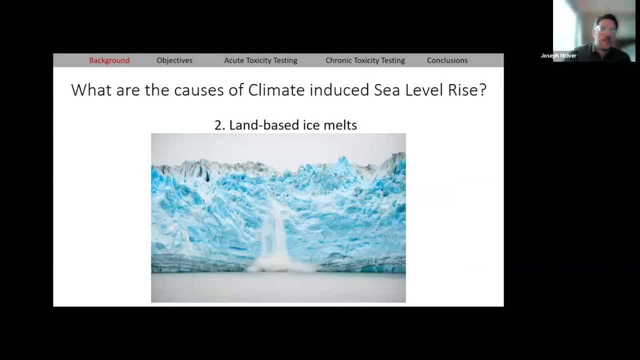 number two is, excuse me, land-based ice melts. so this is landlocked ice that is melting due to, uh, changing climate and it's increasing the volume of water um, in the ocean. so if you've ever filled up a bathtub and turn the tub off, you're ready to go have a nice relaxing. 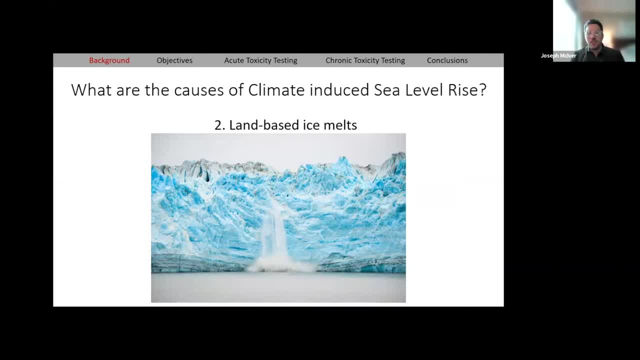 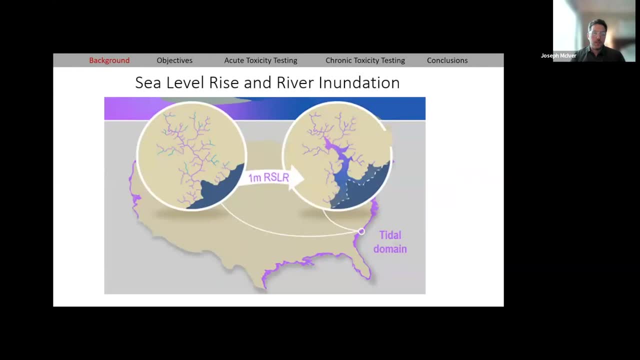 soak, then you get in and that water level rises as you get in. that's the same concept here and as this happens, like I said, the water's expanding, it's increasing, it's going up, it's gonna. it's gonna kind of go to that path of least resistance. so 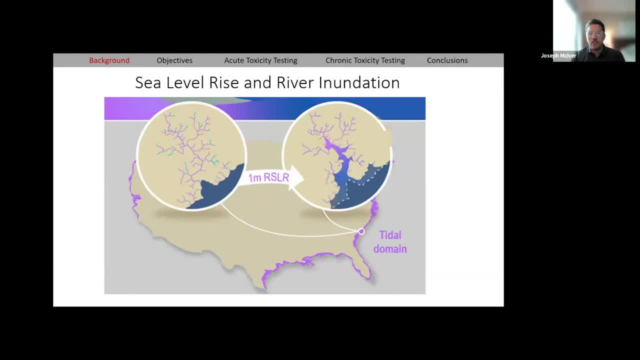 this picture is kind of displaying what could happen in a river system with a meter of sea level rise. so this little circle on the left is maybe what it looks like today, but after a meter of sea level rise you can see that the river is much large, larger at the mouth. so this is the 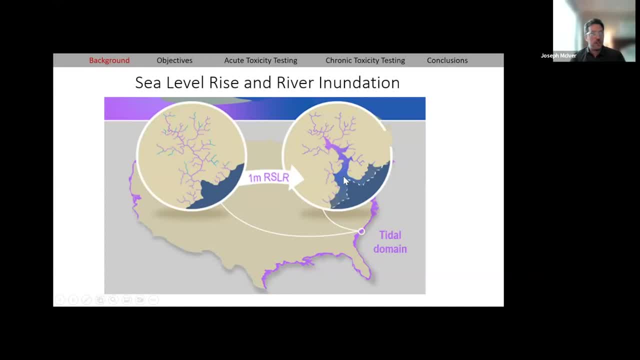 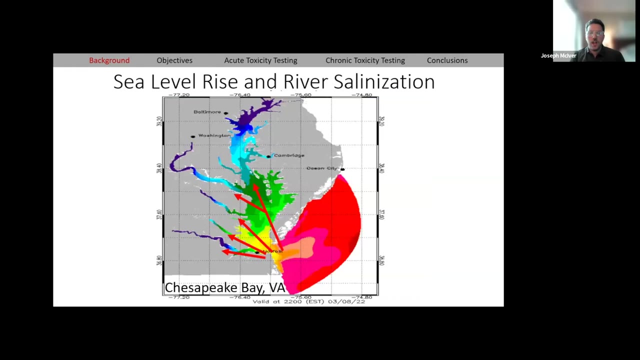 ocean. the river is much larger now towards you know where it meets the ocean. the coast has moved up. so this receding coastline, more water going into the system and reaching further up into these streams and rivers and, as that happens, it's going to carry- sorry, an increased amount of. 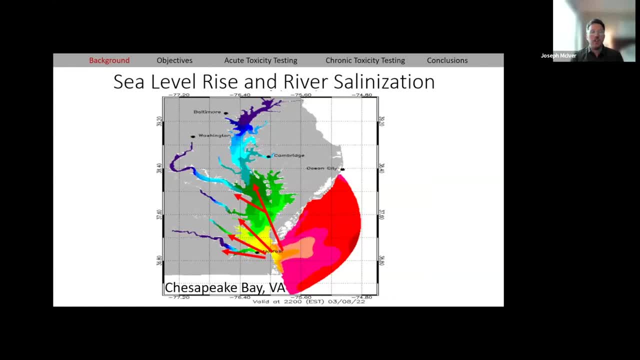 the salt concentration. that ocean is going to bring the salt with it. so this is a photo I pulled off of. there's a real-time salinity tracking system that NOAA has online and you can look at a few different places in the United States and see what the salt content is is at those, at those. 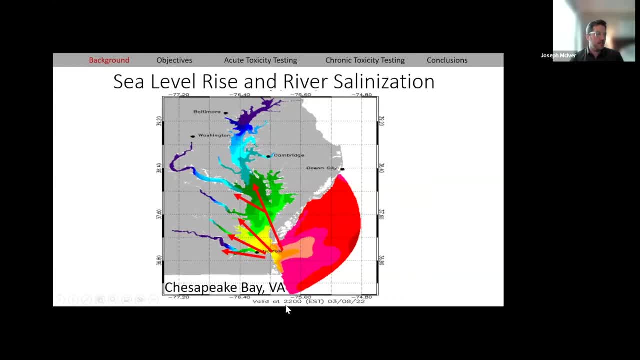 places. so this is Chesapeake Bay. I took this screenshot at March 8th 2022, so about a year ago. and the warm, the colors are high salinity concentrations, so about 34 parts per thousand, going all the way up to these purplish colors around zero parts per thousand. and where it gets into the streams, the 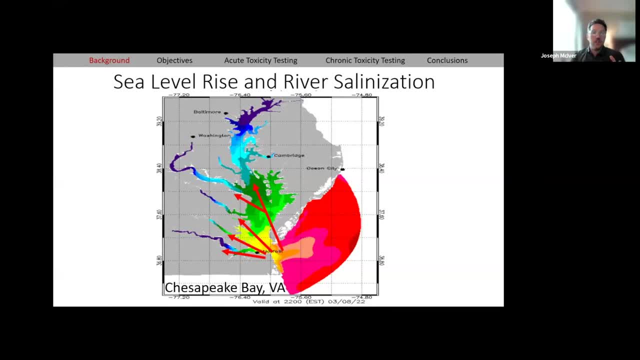 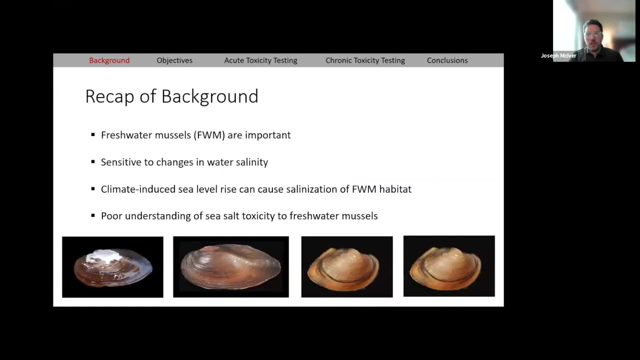 higher parts of the stream down here. so, as that's, as that ocean level increases, it's going to carry that salt with it into these upper reaches of the stream and freshwater mussel habitat. so a quick recap of the background. we now know freshwater mussels are important. I don't know if I stated earlier, but 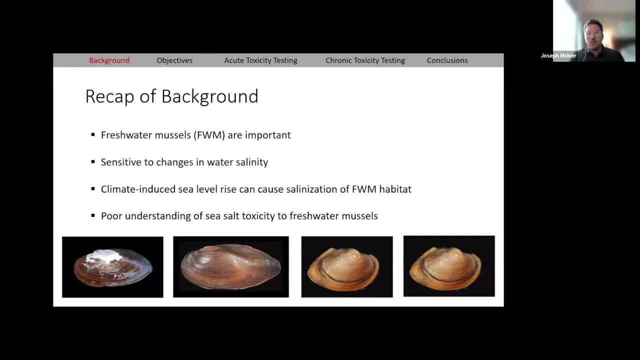 in their feeding strategies. they're always filtering water, so they're a really good source of a water, just a natural living water filter or for us, constantly cleaning our water. they're sensitive to changes in water salinity. climate induced sea level rise can cause the salinization. 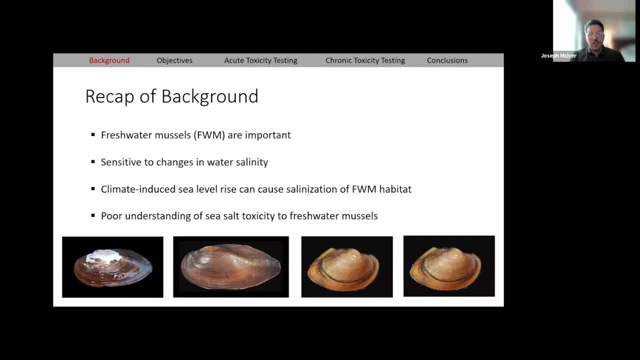 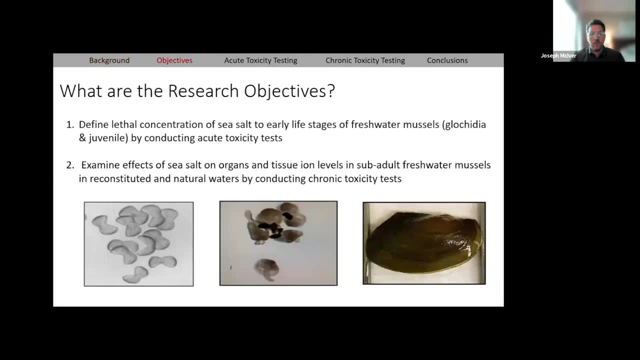 of the freshwater mussel habitat and we don't have a great understanding of of how that, how toxic that is to freshwater mussels. so this brings us to the good stuff. here we're going to get to our research objectives. so, number one: we wanted to define the lethal concentration of sea salt to the early life. 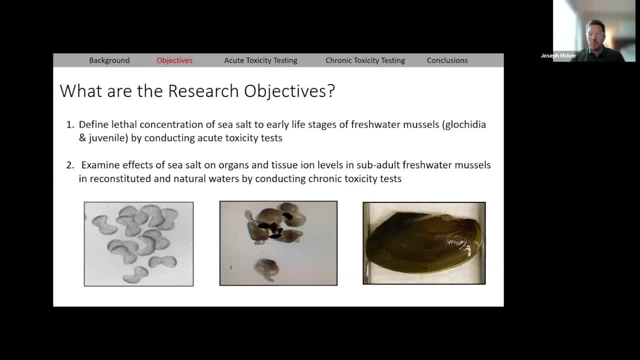 stages of freshwater mussels, so the glochidia and juveniles, by conducting acute toxicity tests. and number two, we wanted to examine the effects that sea salt has on the organs and the tissue ion levels of subadult freshwater mussels. conducting chronic toxicity tests using reconstituted water, which is a, is a lab kind of. 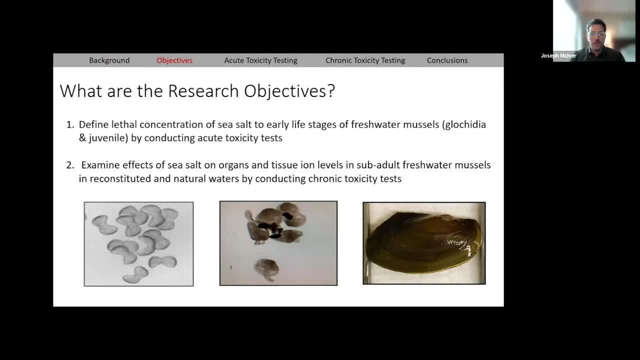 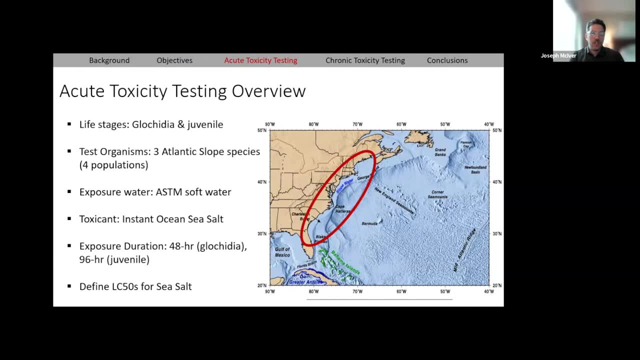 lab made water in natural waters. so first we're going to talk about the acute toxicity test. so this is an overview of that. so life stages. I mentioned glochidia and juvenile. we used three Atlantic slope species so this picture is just kind of saying: generally Atlantic slope is right. 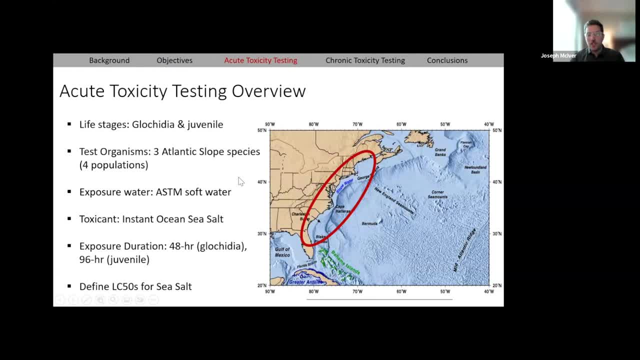 here, so three Atlantic slope species and four populations. we exposed them to instant Ocean sea salt in an ASTM soft water, so that lab reconstituted water, and we exposed the glochidia to this salt for 48 hours and the juveniles for 96 hours. and we wanted. 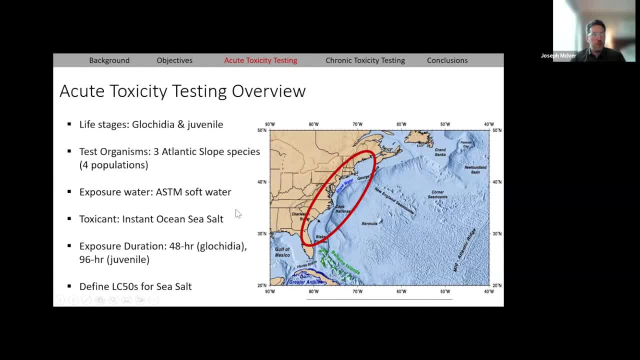 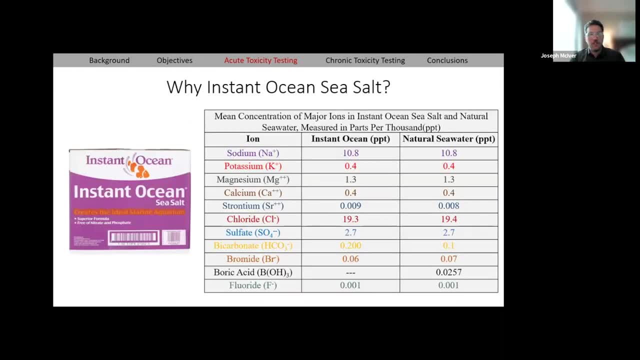 to Define the LC50s for sea salt. so you may be wondering the top about the toxicant instant Ocean sea salt. what? what is that? it's a synthetic formulated sea salt that is made to mimic the, the ionic concentration of natural seawater. so just displaying the different ions. 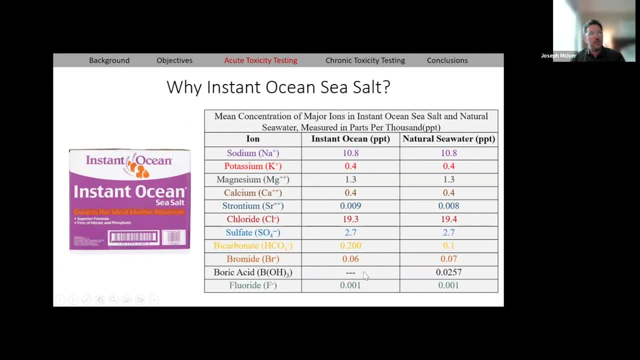 here and their concentrations in instant Ocean sea salt compared to natural seawater they're very, very close, so that's why we chose to do that. there's also some research done on catfish in the Chesapeake Bay area, I believe by Robert bringoff, who used instant Ocean sea salt in. 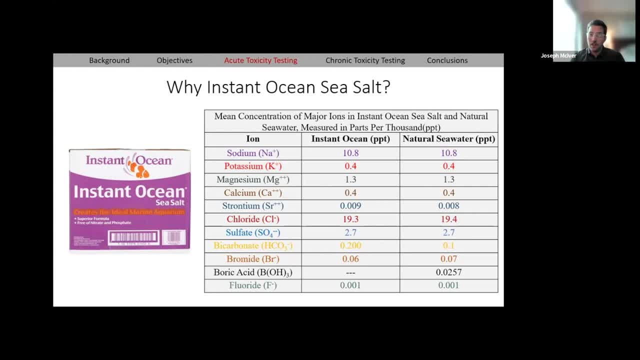 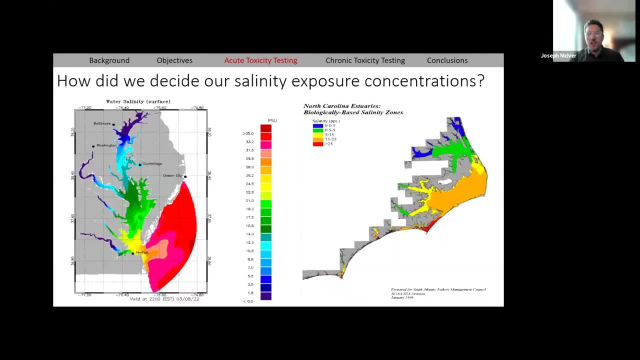 his research as well. so we had a little base of some stuff that had already been done with instant Ocean sea salts. so how did we decide what concentrations of the sea salt to expose our muscles to? so this little photo I showed earlier, we so we looked at the natural. 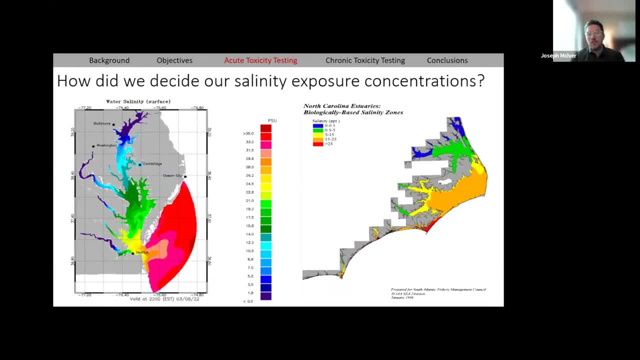 salinity concentrations which are occurring kind of along the East Coast, which range from about 34, 35 parts per thousand, all the way down to zero. so we wanted to expose these muscles to salinity concentrations which they could be could be exposed to due to this salinization of their habitat and those River systems. 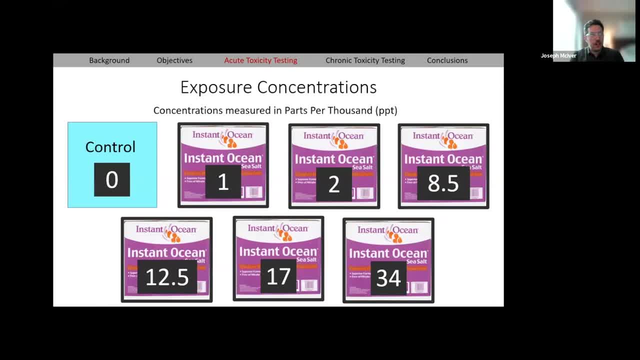 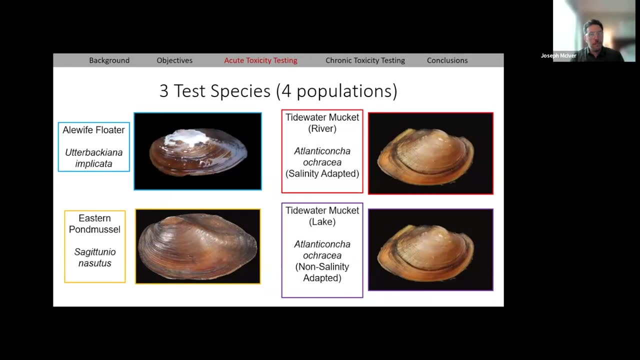 so we chose these six concentrations and a control, so no salt. so our concentrations were one, two, eight and a half, twelve and a half, 17 and 34 parts per thousand. so now we're going to get into our test subjects, our species. here these are our three species and 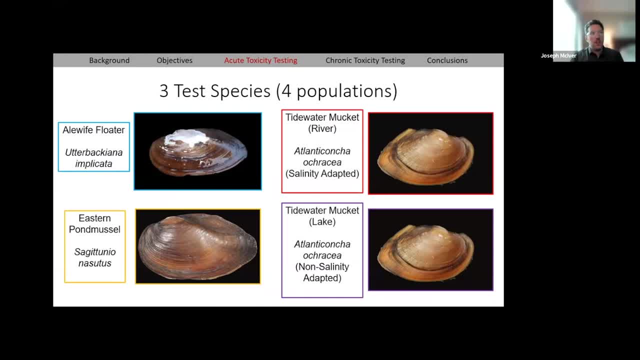 their populations. so the ly floater, the Eastern Pond Muscle, the tidewater mucket from a river population and a lake population. that's where the fourth population comes in. so I will explain what salinity and non-slinging adapted means on the next slide. I believe all 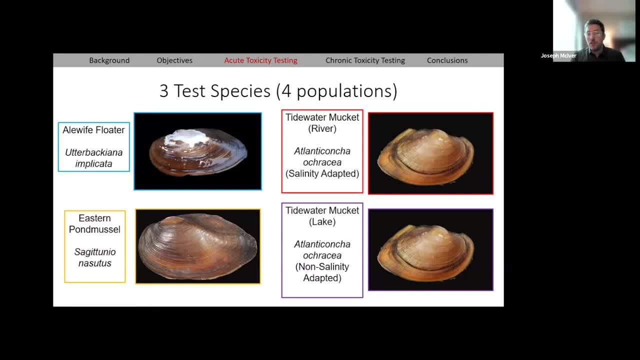 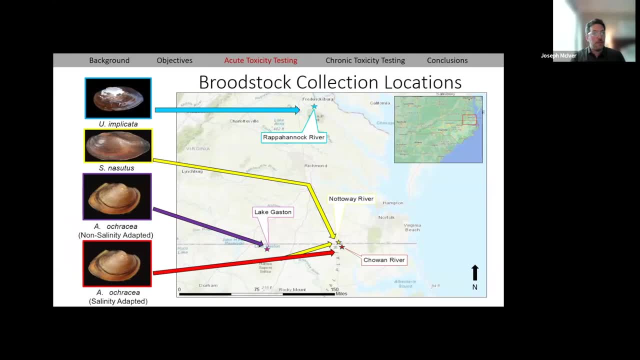 three of these species are listed as threatened in North Carolina. but to get these animals we had to find them and collect them and propagate them. so with the help of the North Carolina Wildlife Resources Commission in the Virginia DWR we went out and collected the gravid females. so these are. 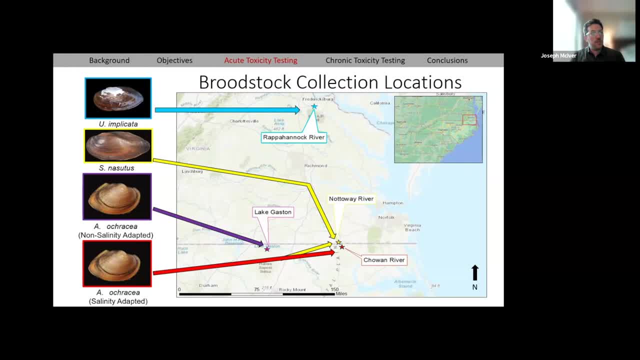 the pregnant female muscles. so we collected them from these locations and then we transported them to Harrison Lake National Fish Hatchery, which is around this area just outside of Norfolk, Virginia, where they were propagated. so that's where the glochidia and the juveniles were produced. and then, when it was time to conduct our toxicity, 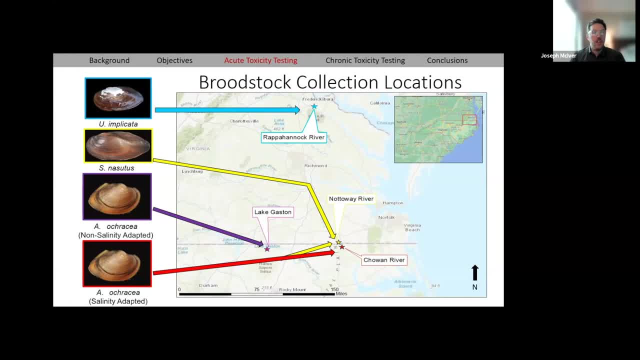 test. I went up there to the hatchery and brought them back to NC State. so let me, let me explain this non-salinity adaptation and salinity adaptation thing. so this is sort of a hypothesis you can think of it. salinity adapted in quotes: okay, so these salinity adapted. Atlanta, concho-ocracia. 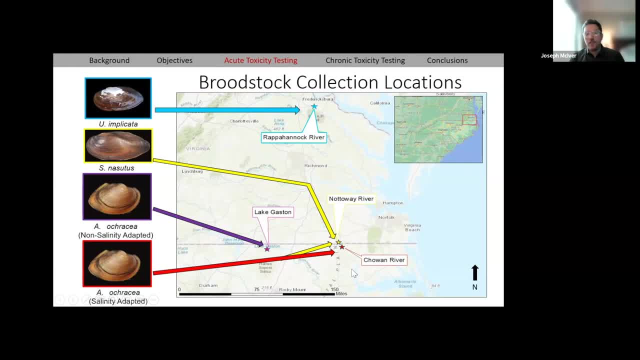 they were collected from the Cho Juan and Nottoway River which experienced a natural exposure to salt. So I know in the Chowan River near our collection site, there has been documented levels of four parts per thousand of sea salt near those collection locations, Whereas the Atlanta, Concha, Ocratia from the non-salinity adapted ones are from Lake. 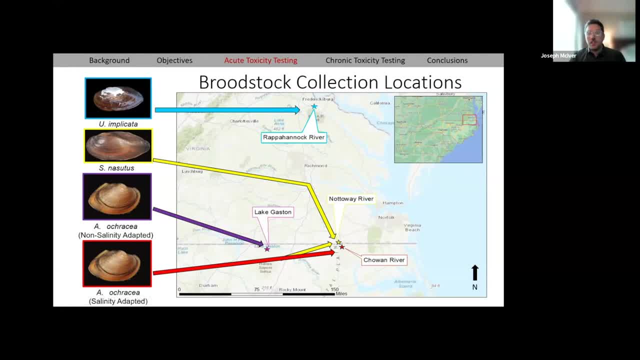 Gaston Lake. Gaston has been cut off from the river, so it's a dammed reservoir. It's been dammed, I think, since the 1960s, So there's been about 80 years or so where there's been no ability. 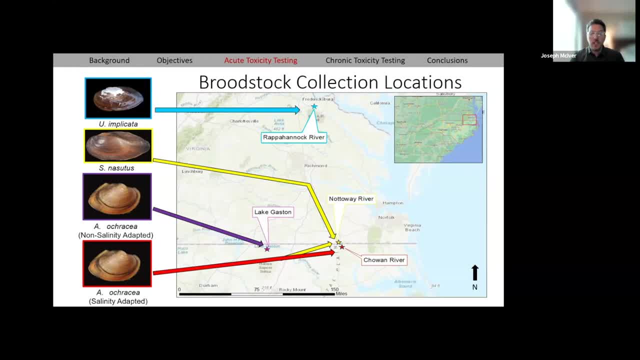 for any salt to get into that, into that lake, or any mussels from a lower reach of the river to get into that lake. So any possible salinity adapted mussels- since they need fish to reproduce- the glochidia can get hooked onto the fish and the fish then could get into the lake. 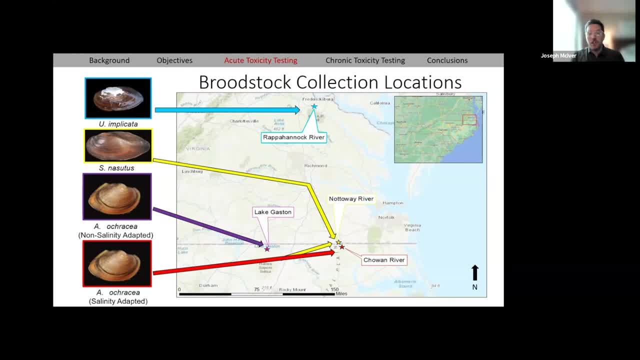 and those mussels could come from a more salinity exposed place. But since it's been dammed there's been no ability for those mussels to get into that system. So that's kind of a hypothesis, thinking that the salinity adapted mussels would have. 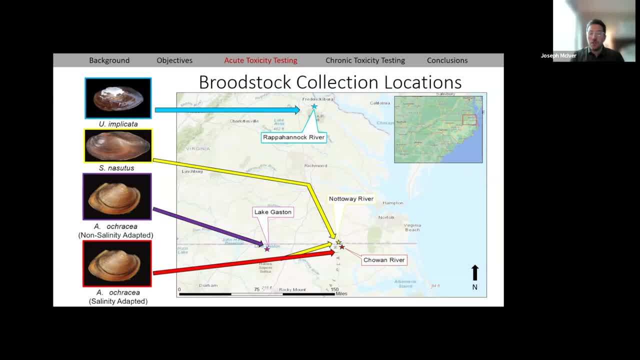 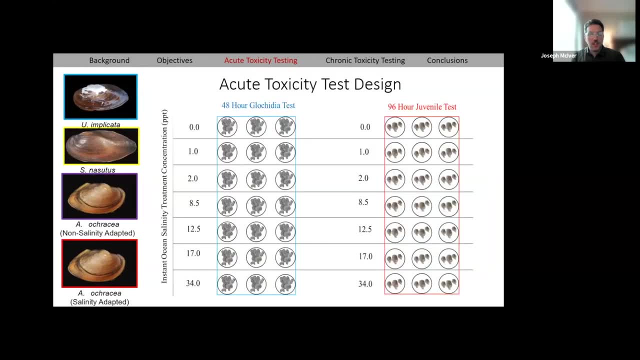 a great greater ease of dealing with the salt than the non-salinity adapted, So we kind of wanted to look at that as well. So now the acute toxicity test design. So each of the four mussels on the left there. we conducted a 48-hour glochidia test and 96-hour juvenile test. I'm exposed. 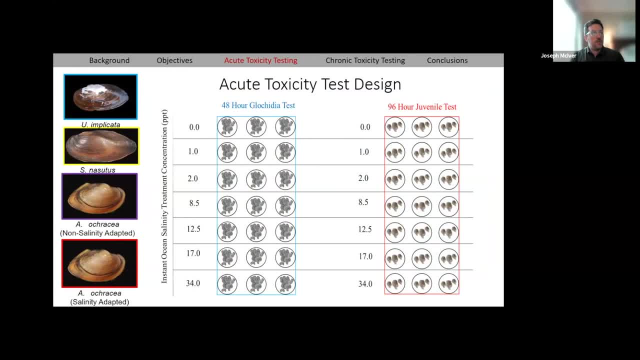 them to those concentrations of sea salt ranging from 1 to 34 parts per thousand. For the glochidia, we measured survival at hour 24 and hour 48, and for juveniles we measured survival at hour 48 and hour 96.. Within the glochidia test, each treatment level so 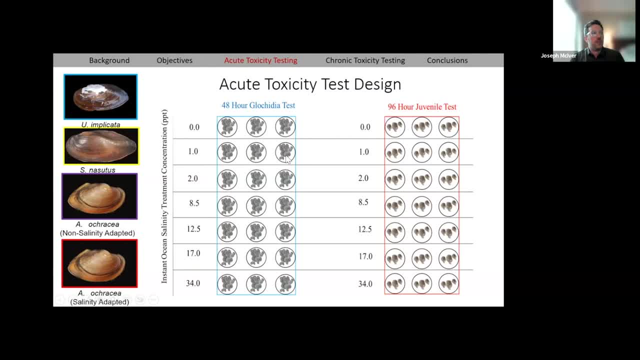 each salinity concentration, there were three replicates within that concentration, And each little dish here contained about 250 mussels with the glochidias juvenile test. Once again, each treatment concentration consists of three replicates, except this time there were about 10 juveniles in each replicate. So now we get to the results. 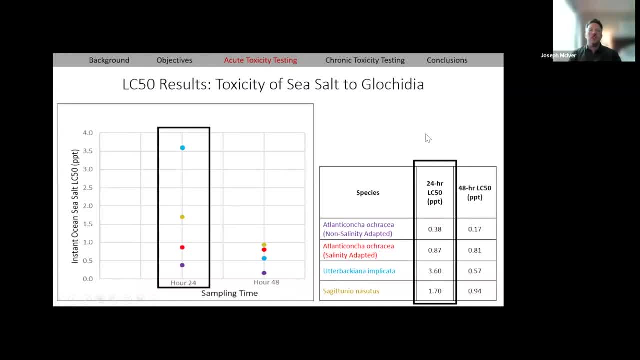 So these are the LC50 results for the toxicity of sea salt to the glochidia mussels. I have outlined here the 24-hour LC50 because, as I stated earlier, that's the time point that the EPA uses for their water quality criterion And we found that the LC50s range from about. 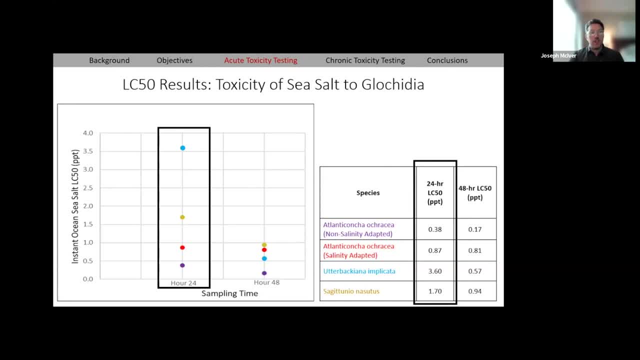 0.3 parts per thousand to three parts per thousand and that the non-salinity-adapted- Atlanta, concha, ocratia- were the most sensitive to sea salt. Just for fun, the 48-hour LC50s. so right here you can see the numbers decreased the longer they were exposed to the sea salt. 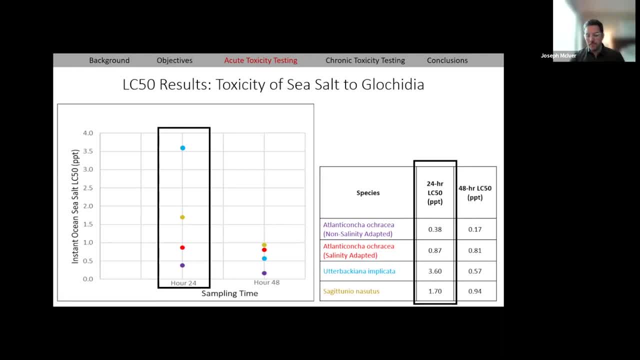 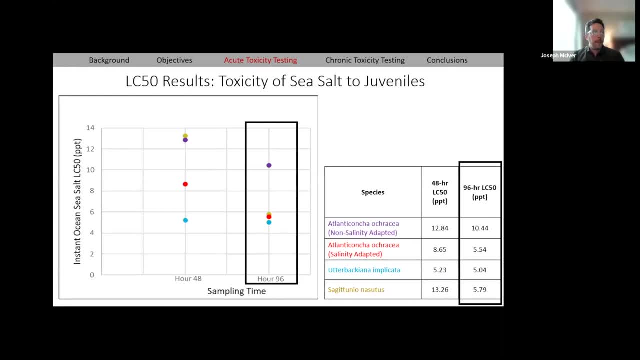 just meaning. the longer they were in it, the more toxic it became to them. Now for the LC50 results for the juveniles. So once again, the black box denotes the time point the EPA uses to set their water quality criterion, and for juveniles it's hour 96.. 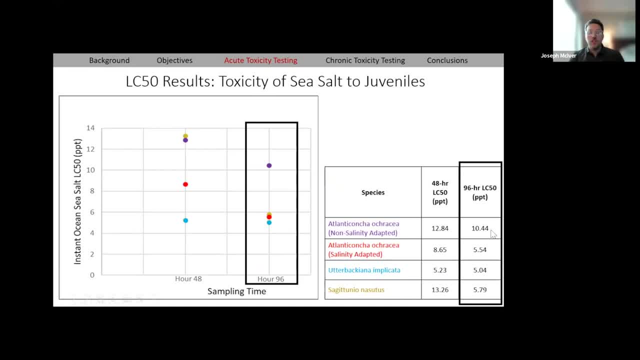 Those concentrations range from about five to 10 parts per thousand And, in contrast to our hypothesis, the non-salinity-adapted Atlanta, concha, ocratia were now the most tolerant to sea salt. So you can ask for the LC50 results for the juveniles And once again the black box denotes the length of the LC50s range from about four to 10 parts per thousand, And for juveniles it's hour 96. So once again, the black box denotes the time point the EPA uses to set their water quality criterion. just meaning the non-salinity-adapted Atlanta, concha, ocratia were now the most tolerant to sea salt. 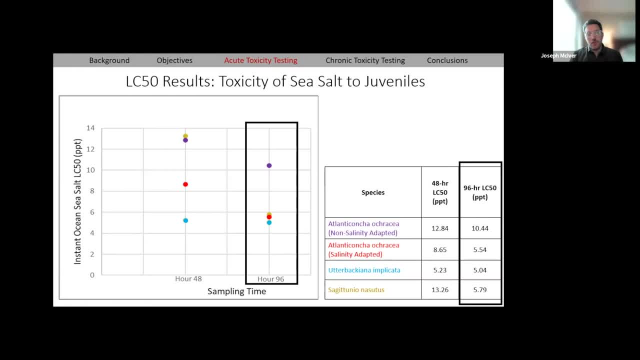 So once again, the black box denotes the time point the EPA uses to set their water quality criterion, And I unfortunately won't have an answer about why that is. I would love to look into that more and run these tests again and see what we get. It's just a fun little nugget and we don't know. 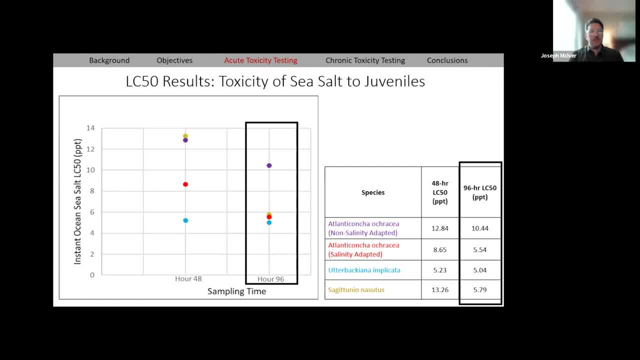 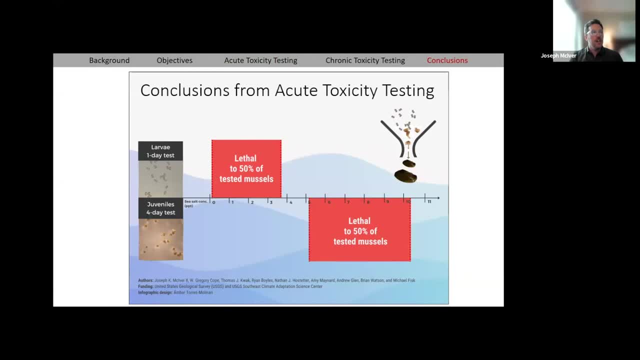 what happened or why, but yeah, so I'll continue. So our conclusions: from the acute toxicity test, we found that these lethal concentrations 0.3 to 3 for glucidia and 5 to 10 for juveniles. The main thing I want you to take away here is that the glochidia were the most sensitive. 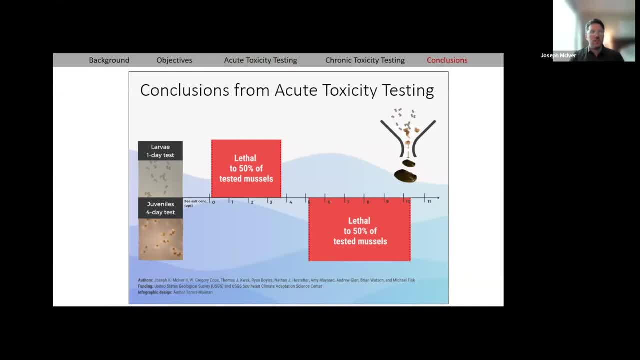 life stage to this sea salt, kind of representing a reproductive bottleneck: If your glochidia are dying, you're not going to get juveniles and you're not going to get adults. And I'd like to thank once again Seacask and the designer, Ambar Torres-Morinani, and 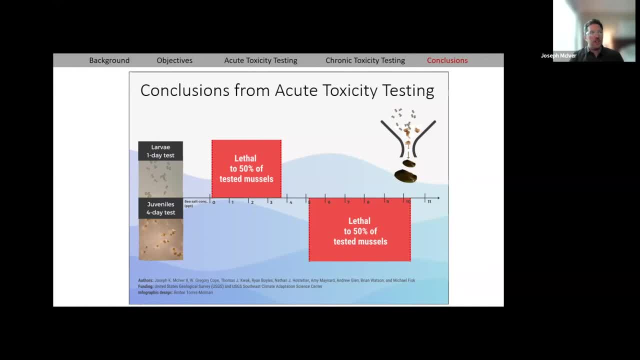 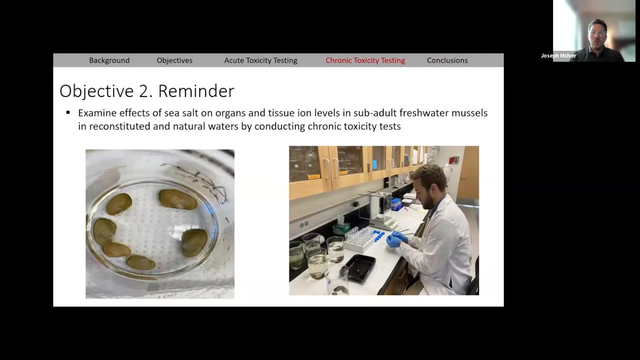 all of the authors who put a lot of work into this really great infographic. I think it does a great job of kind of displaying the conclusions from that acute toxicity test. So now a little reminder. we're going to move into objective two. We wanted to examine the effects of sea salt on the organs and tissue ion levels of the. 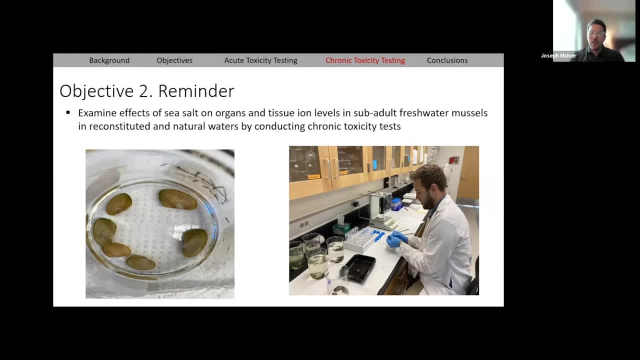 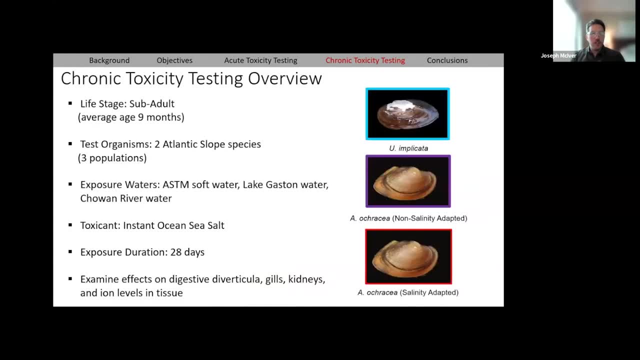 subadult freshwater mussels in the reconstituted and natural waters by conducting the chronic toxicity tests. So a little overview. These were subadult mussels. Their average age was about nine months. The test organisms, so those species, are on the right, the Uterbeckia and Implicata, and the two 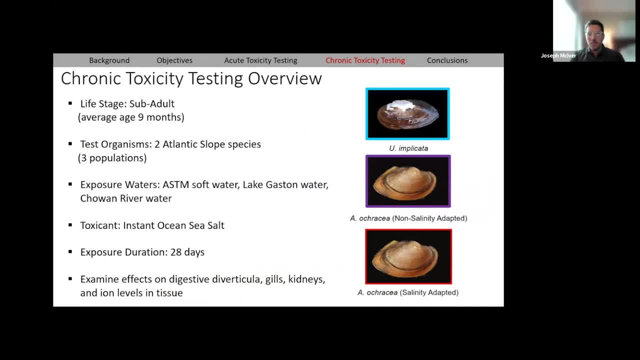 Ocratia populations. We exposed them to the same toxicant that instant ocean sea salt, but this time we put them in ASTM soft water, Lake Gaston water and Chowan River water And we exposed them to this toxicant for 28 days and we wanted to examine the effects on their 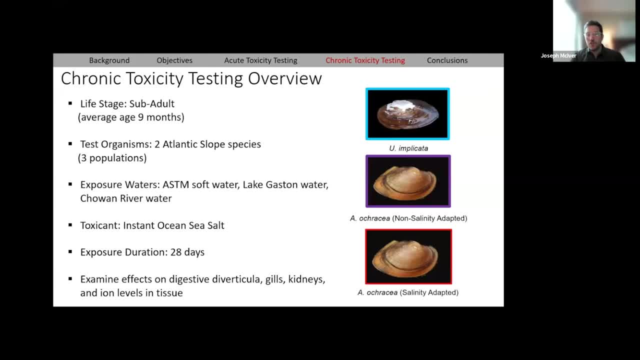 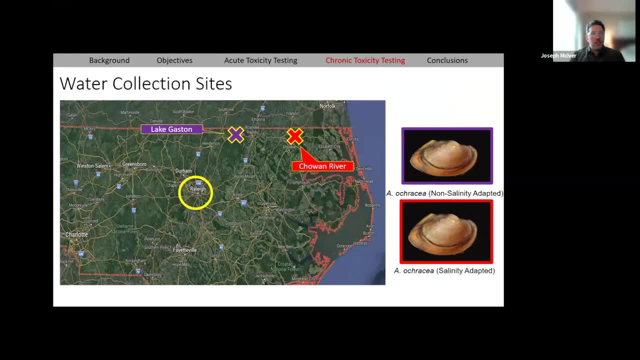 digestive glands, their gills, kidneys and the ion levels within their tissue. So, Being that we use natural water for a couple of these tests, that was a big hurdle with this part of the research. So, us being in Raleigh, we had to, I think, once a week go out to the Chowan River and Lake Gaston. 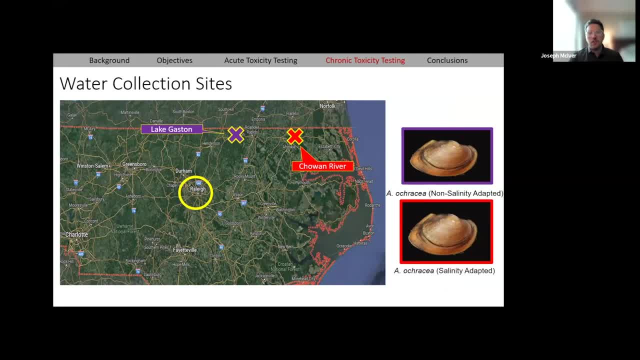 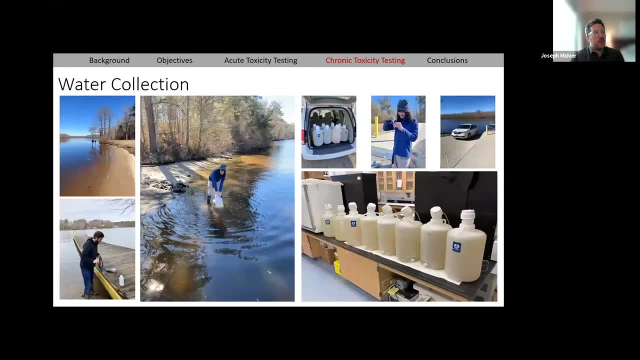 to collect water to run these tests, So I think it was a whole day affair and a lot of driving time to go get this water. So this is some photos from. Here's some photos from all of that fun. This man is Clayton Lynch. 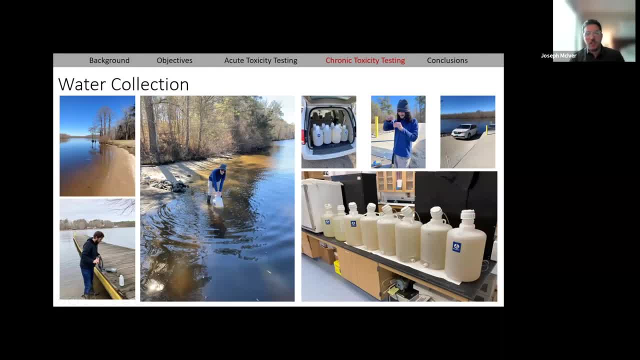 He was my technician at the time, who's now a graduate student at NC State University, And he bared my presence for that time and he did great work, So I want to thank Clayton. Once we collected the water, we put it in the van and this is what it looked like in the lab. 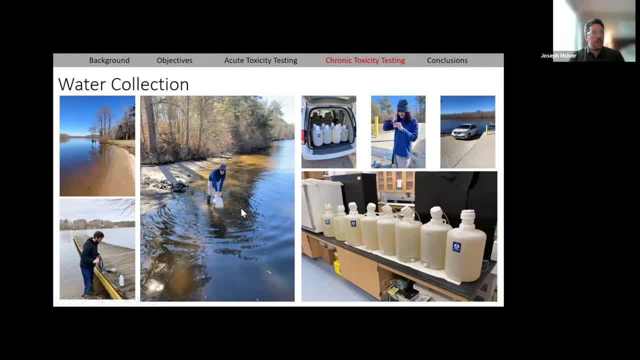 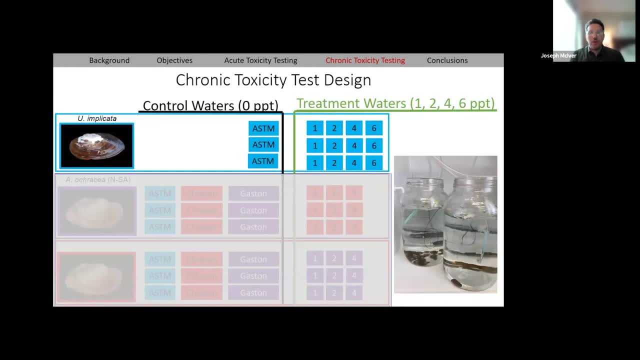 We got it back to the lab where we could use it for our toxicity tests. So the design of our, Our chronic toxicity tests. I'm going to break it up into two little pieces here. First, I want to point out the Uterbachiana Implicata test. 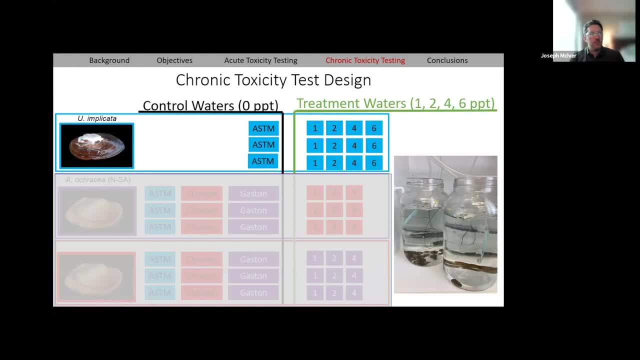 So this was conducted in just the ASTM reconstituted water. So each one of these boxes here represents a jar of mussels. Each jar had about 10 to 12 mussels in it. So we exposed Uterbachiana Implicata to these four concentrations of instant ocean sea salt: one, two, four and six. 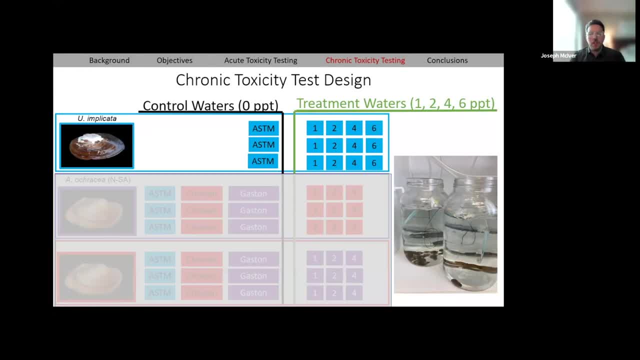 In that reconstituted water And we sampled them for the organ tissue organ analyses and the ion tissue analyses at specified time points, which I'll get into in a second. We also took baseline samples for comparative purposes. So those were mussels that had not entered into any salt. 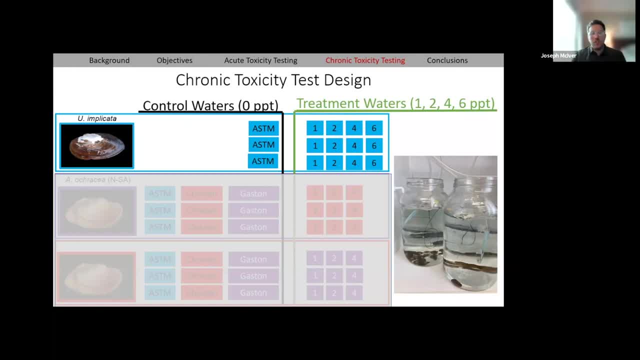 So we could say, hey, you know, these mussels are what's supposed to be a healthy looking gill compared to a mussel that had been in the six parts per thousand. But we want to make sure that they're not in the water or in the sea salt. 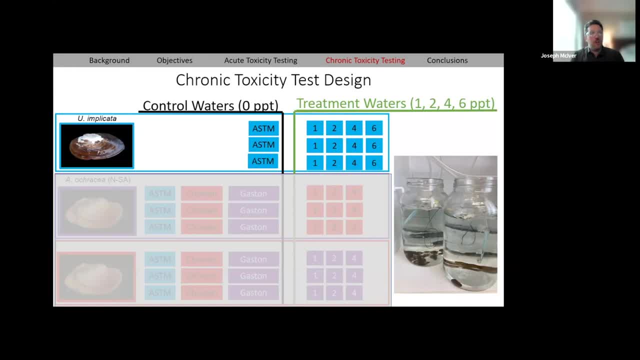 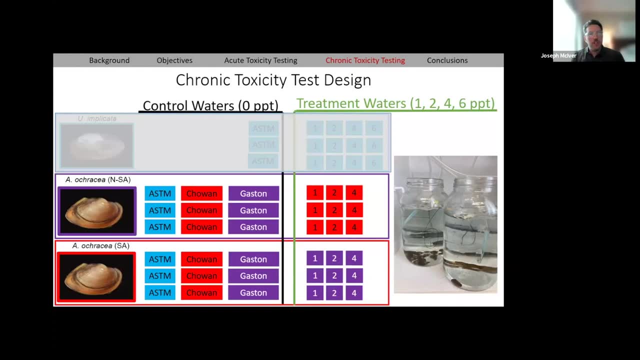 This is what it looks like compared to a nice muscle, a nice, healthy muscle. So just wanted to clarify that. next, We conducted these two tests. We did them at different times, but I wanted to show them together because it makes sense. So, the non-slim adapted Ocratia week: we exposed them to. 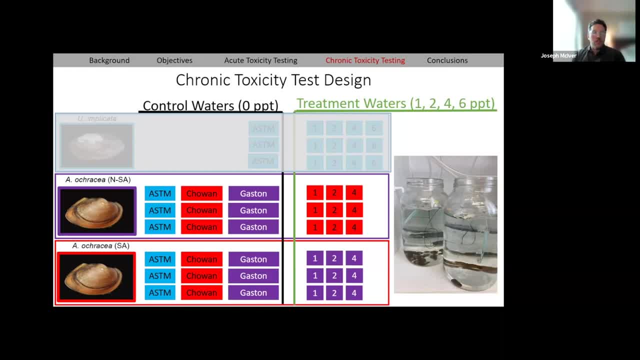 So they're from the lake, We expose them to salt. In the river water, We exposed them to salt and vice versa for the salinity adapted ocratia, so we exposed them to salt from it within lake water, being that they're from the river. so we kind of wanted to get at a kind of reciprocal. 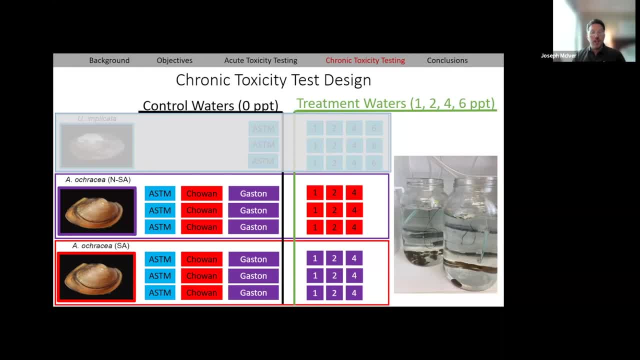 transplant experiment. so if you can think of, maybe you put lake mussels in the river and river mussels in the lake in a natural setting, how would they fare when they're exposed to salt? so that's what we were getting at here, and we did not expose them to six parts per thousand of sea salt and 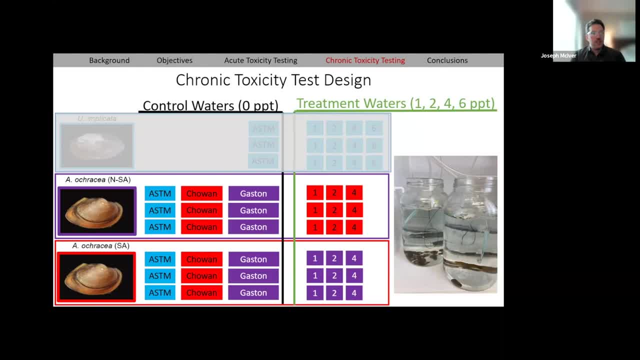 i'll get into that in a minute- and kind of the reason behind a reciprocal transplant experiment was maybe there needs to be some augmentation of the populations in the future, so maybe if some of the mussels in in the river get exposed to sea salt and they die off, can we use these lake mussels. 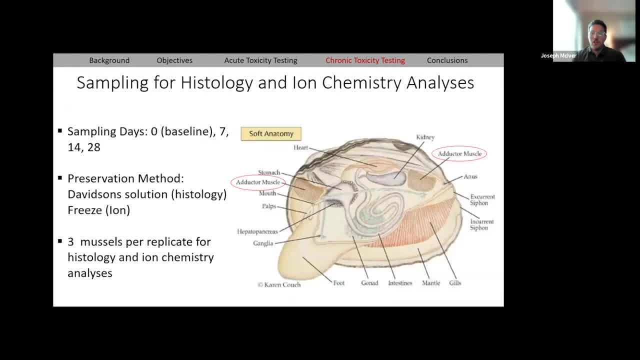 to replenish that population. so now i want to get into the sampling for the systology, the organ, organ tissue analyses in the ion chemistry analyses. so we say, sample these mussels at the baseline, so day 0, 7, 14 and 28, and then we preserve them in davidson. 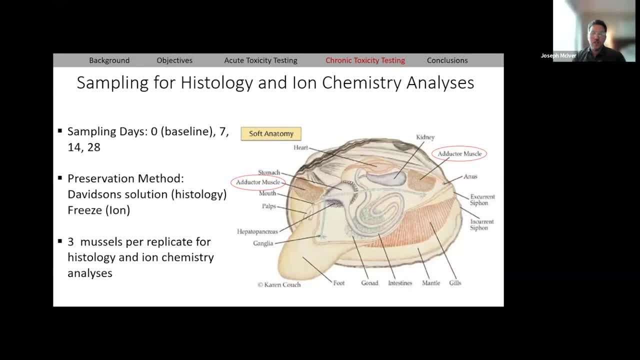 solution for histology for one to two days, and then we transfer them over to 70 ethanol and then for the ion tissue analyses we just froze them at negative 20 degrees. we did that for three mussels per replicate, for each of the sampling and each of the analyses. so for the histology and the ion, 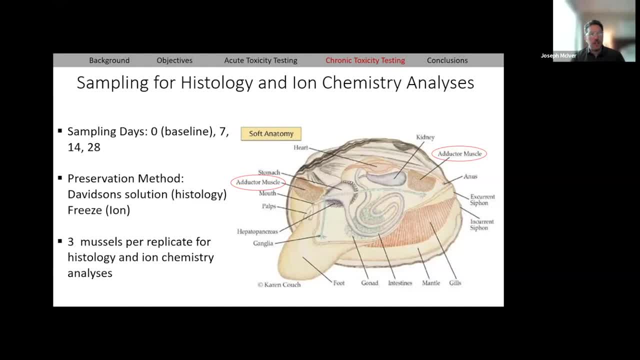 chemistry analyses. so we did that by um. essentially, this is a glorified oyster bar, um. so we shucked the muscles by severing this adductor muscle right here um the anterior and posterior adductor muscle. once you do that, the muscle will release and open up and it will allow you to carefully take out um all of. 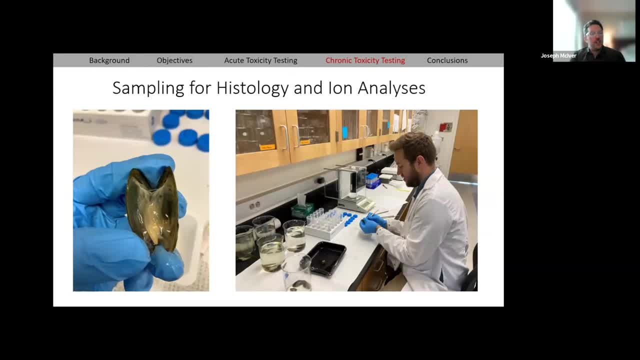 that body tissue in there. so this is a a process of that happening. um, very, very smelly process, but uh, it's good. so after we sampled it, sampled these muscles, we sent them off to, uh, frank weber at rti, who conducted our ion chemistry analyses, and talvin horan, um, who's at nc state. 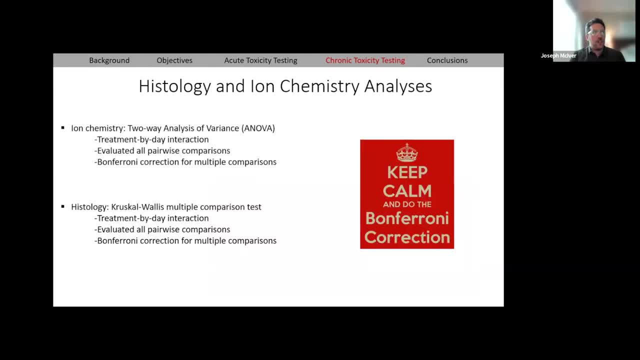 who conducted our a um the histology analyses and these are the statistics we ran for those various tests. so we ran a two-way anova for the ion chemistry and a cruz school wallace multiple comparisons test for the histology And we used a Bonferroni correction for all of those comparisons and crazy p-values we got. 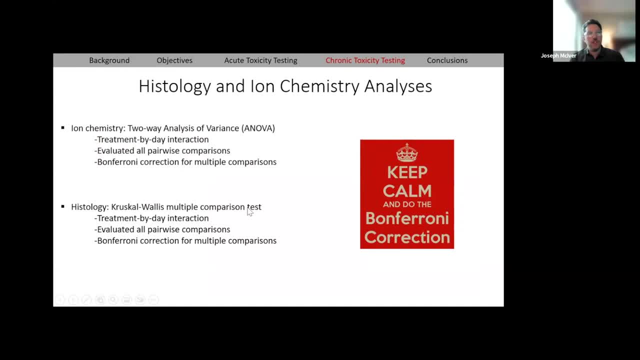 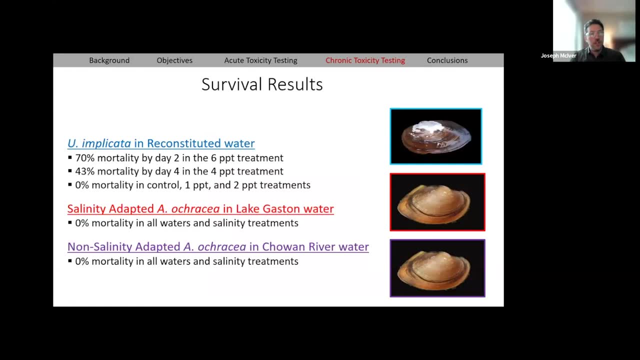 So hence the keep calm, Bonferroni fixes everything. Okay, so now we're going to get into our results. So we had some really, really interesting survival results. with this chronic toxicity test For the Uterbacchia implicata, we found these muscles exhibited a lot of mortality. 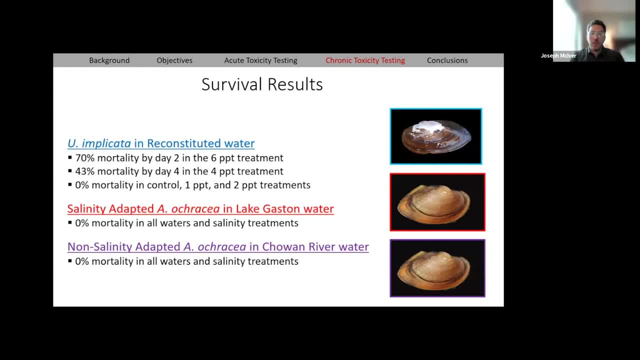 70% by day two of the test in the six parts per thousand treatment and 43% mortality by day four in the four parts per thousand treatment. And there was no mortality in the control one or two parts per thousand treatment. So these were muscles exposed to the salt in the reconstituted water. 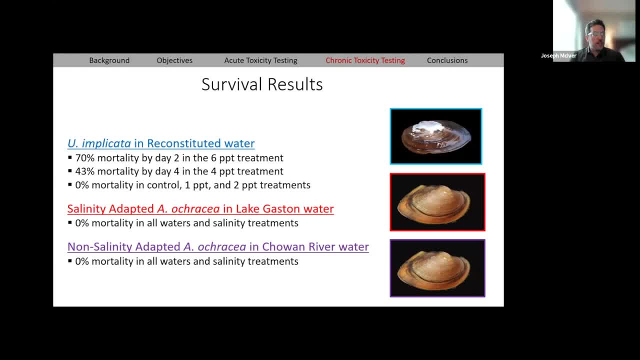 For the Ocratia, each Ocratia test. they exhibited no mortality in any of their exposure. So that's That's why I didn't. We didn't want to expose them to six parts per thousand of sea salt, because our goal was not to 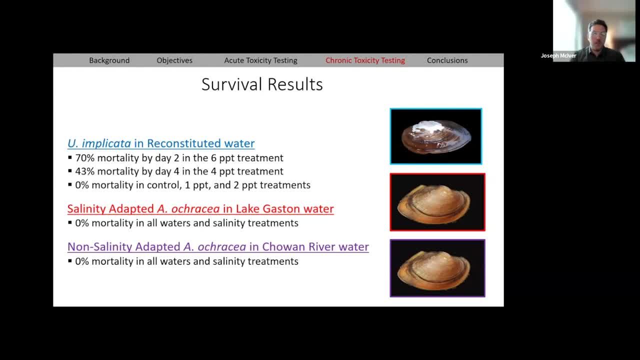 Really we didn't want to kill these muscles before it was time to sample them because we were trying to get at those sublethal effects And we think this was really interesting, that the muscles in the natural water they didn't experience any mortality, even in the four parts per thousand treatment. 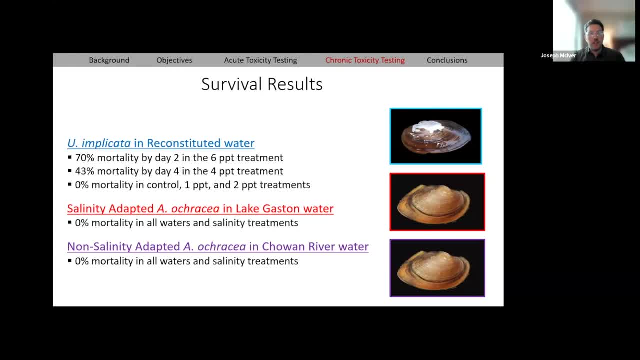 So we're thinking that maybe there is some protection they're receiving from being exposed to salt in natural water. Maybe there's some binding going on with the salts and the carbon, the dissolved organic carbon, in the system There's also- There are also different species here. 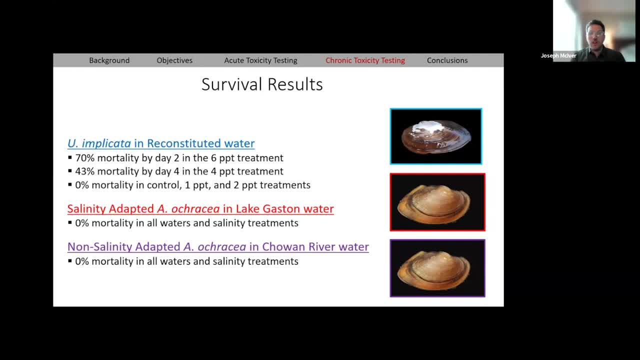 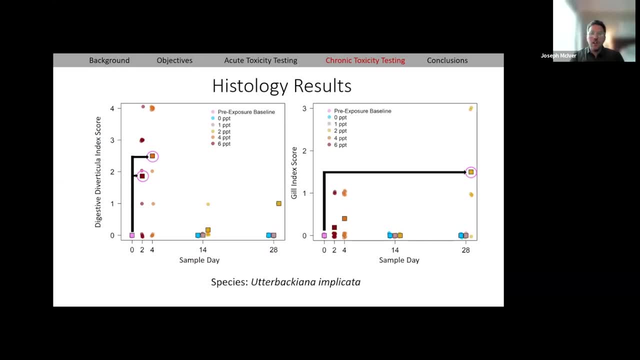 So there's some really, really neat results with this right here that I'd love to see more research done on that. So now getting to the histology results. So looking at these organ, These effects on the organ tissues- This is for the Uterbachia implicata. 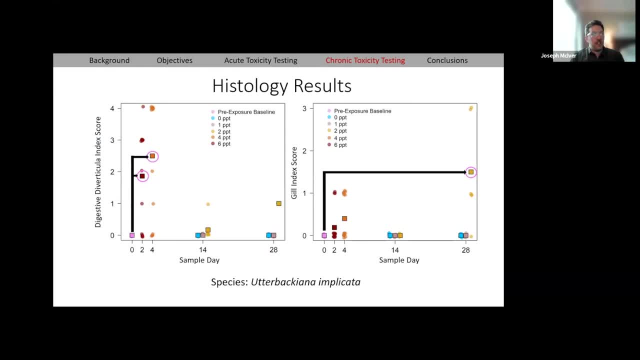 The box on the left is for the digestive, The digestive system. in the box on the right is for the gills. The x-axis is the sample day And the y-axis is an index score. So the greater the damage done to that organ system, the higher score it received. 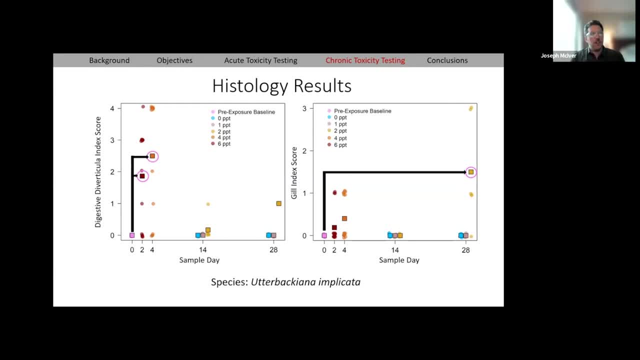 Each little point you see, there is an individual sample And the box you see is the mean of samples within that treatment. So what we found here is kind of what I'm pointing out with the arrows and the pink circle. So we compared, We compared the means to the baseline mean, which is that pink square at day zero. 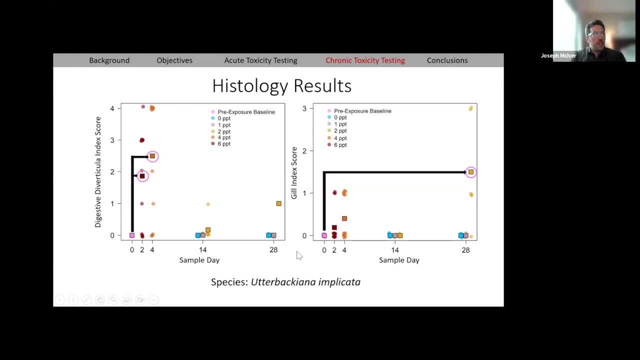 And we found that the Uterbachia implicata that was exposed to six parts per thousand of sea salt and four parts per thousand of sea salt at those sample days They had a significantly greater amount of damage done to that digestive system than the baseline muscles. 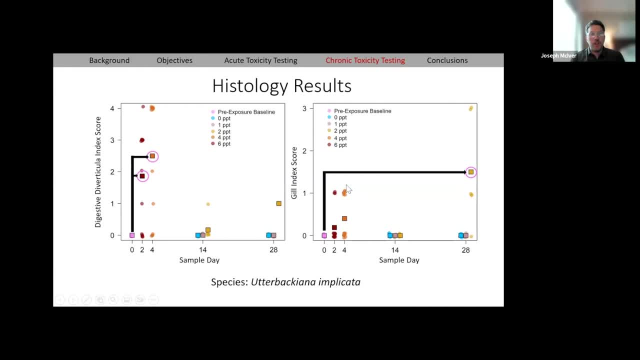 On the gill system. there was a significantly greater amount of damage done to the gills than to the serum, the Uterbeckia amplicata, at day 28, in that two parts per thousand of treatment. So it's kind of. 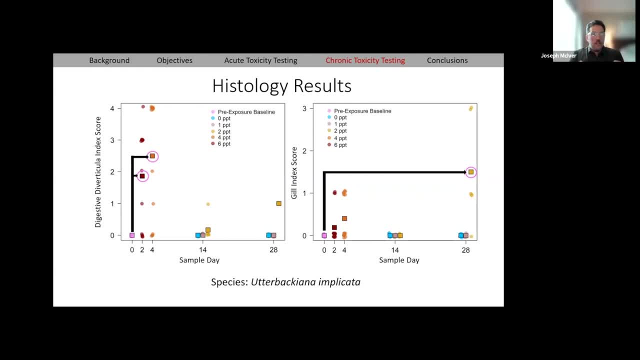 like the fast, quick, hard. high exposure to sea salt impacted the digestive system very heavily. We think that's why the mortality occurred. But these muscles that got to stay in the salt for longer, it looked like it was taking some time and it would mess with their gills, So that kind 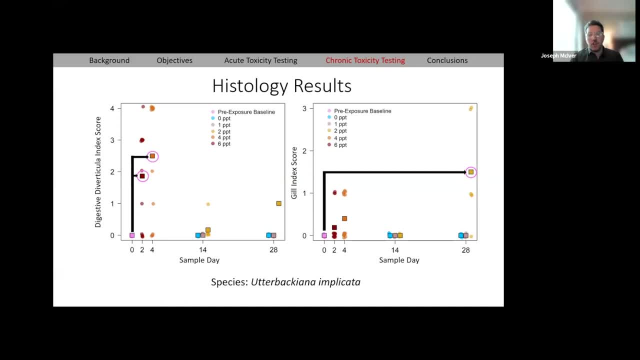 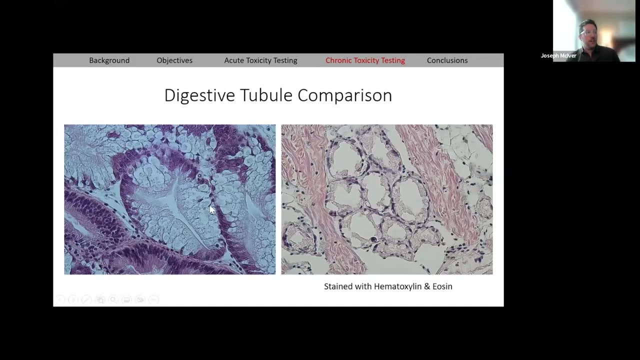 of goes back to some of the research I talked about in the background where it can impact their respiratory system. So I think that's a really cool finding we have with this research. So this is a comparison of those digestive tubules. So the picture on the left is a healthy. 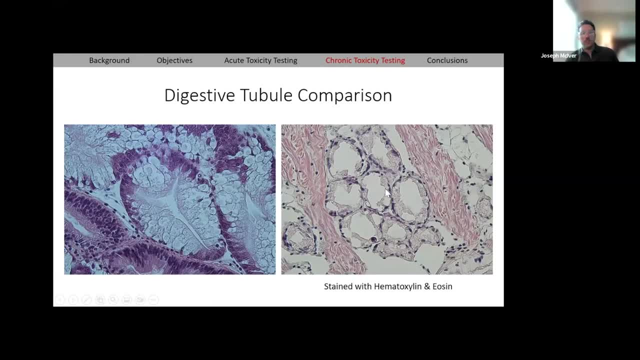 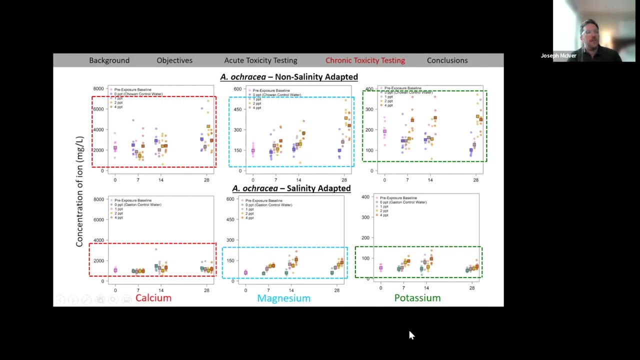 good muscle digestive tubule. And the one on the right is what ours looked like after exposure to those four and six parts per thousand of sea salt. So it essentially got dissolved very, very quickly when exposed to the salt. Okay, so this is a lot of information. We'll figure it out. It's not going to be hard, I promise It'll. 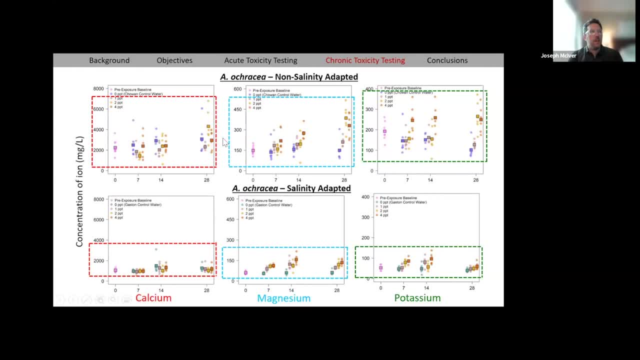 be painless. But this is comparing the ion, so the ion tissue ion concentrations for the elanocontraocratia, the non-salinity adapted, these three boxes on the top with the salinity adapted ion concentrations for the ocratia on the bottom. So we're looking at calcium magnesium. 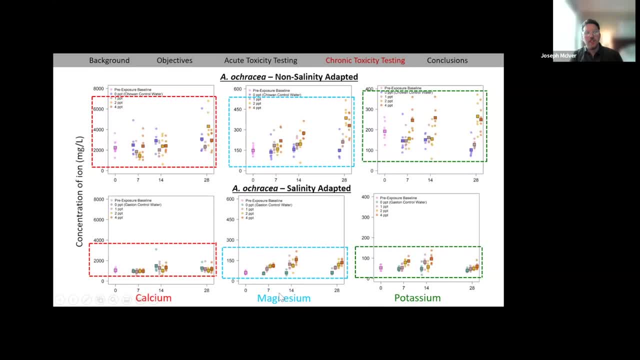 and potassium. The x-axis is the same, It's the sample day, And the y-axis has now changed the concentration of that ion. So what I really wanted to display here is just the range of values compared between these two populations. So all of the little points are so spread out with the non-salinity adapted ocratia, They're 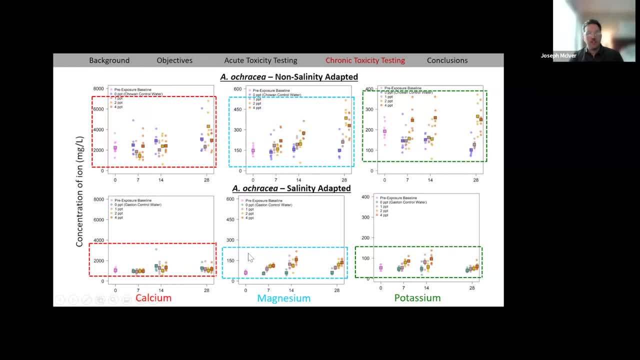 so spread out around the boxes, around the means, compared to the salinity adapted ocratia where these points are much more tightly packed around those. I think that was the big takeaway from the ion tissue analyses. It just kind of looked like the 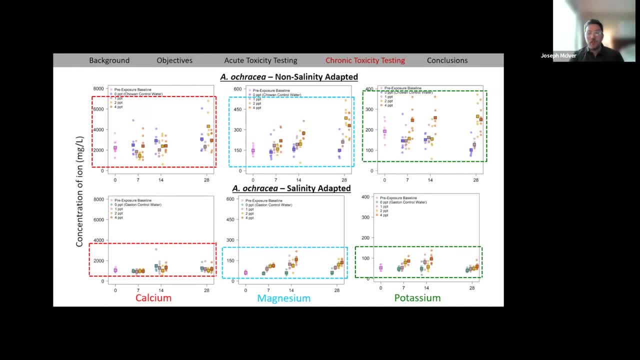 non-salinity adapted ocratia were having a more difficult time regulating their internal ions, bodily ion composition and levels compared to the salinity adapted ocratia. So I thought that was very, very interesting. So now we're getting to the conclusions. 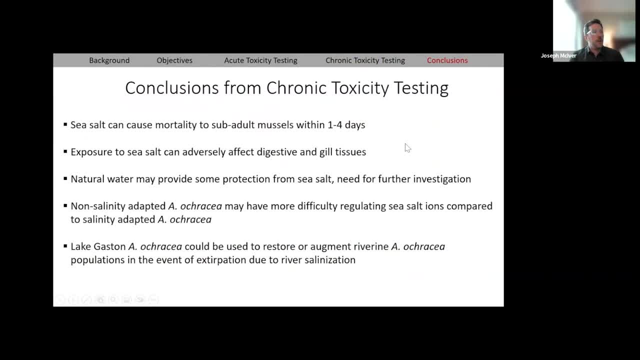 Of the chronic toxicity tests, number one: sea salt- can cause mortality to these sub-adult muscles within one to four days. The sea salt can adversely affect their digestive and gill tissues. That natural water may provide some protection. I'd like to look at that more. There's a study. 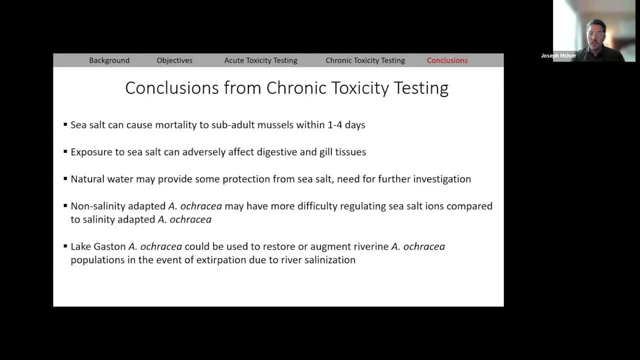 by Gillis 2011, who looked at that with glochidia, and she kind of found the same thing: that these muscles were more tolerant to sodium chloride, So the salinity adapted ocratia can cause more mortality to these sub-adult muscles in the same way. 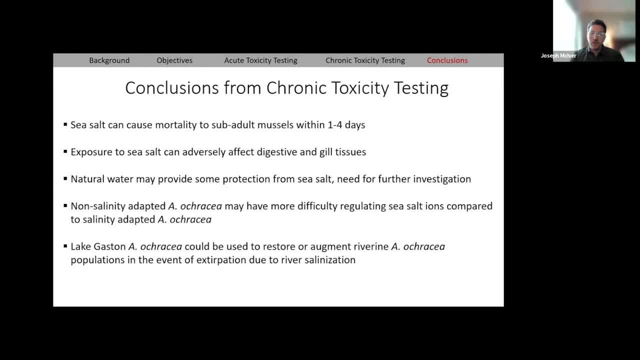 That's what we're working on. We're working on the salinity adapted ocratia. The salinity adapted ocratia have a little bit more salinity. They're a little bit more tolerant to the natural water compared to the reconstituted water. 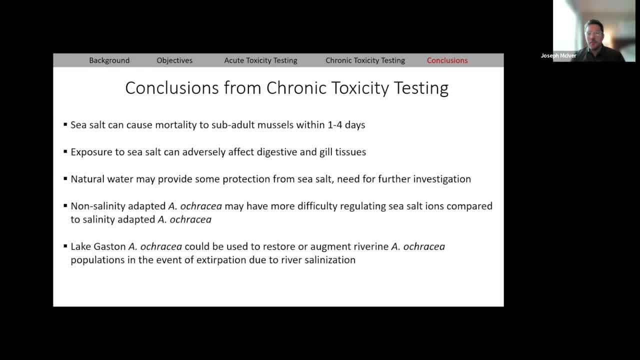 but I think it'd be awesome to keep looking at that. We found that the non-salinity adapted ocratia may have a more difficult time regulating those sea salt ions compared to the salinity adapted ocratia and that the lake gastin ocratia. so those are the non-salinity adapted. they could be used maybe to restore, augment the riverine populations. 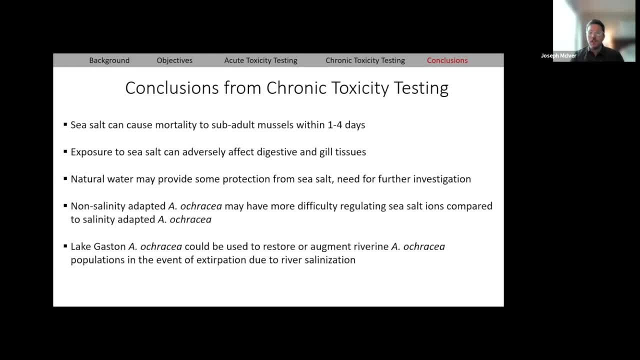 of the salinity adapted ocratia in the event of expertise and environmental damage. And then we're looking at what's going to be the next step in that process. event of exportation, excuse me, when mussels die in the lower reaches of river due to. 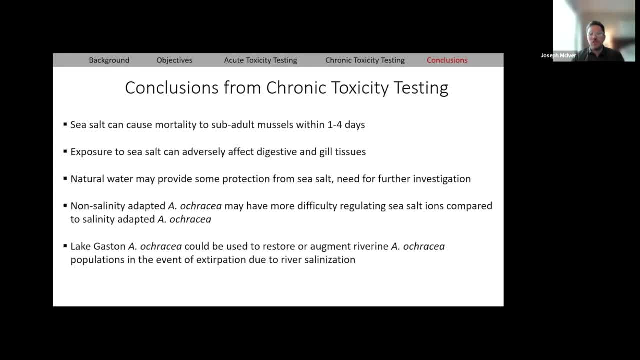 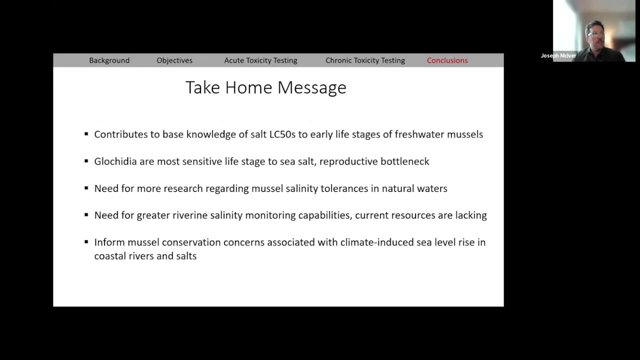 salinization, simply because they survived in those chronic toxicity tests when exposed to that sea salt. So if necessary, they could be used to help for some conservation concerns there. So this kind of brings me to the take-home message. Um, so we think that this research contributes to a base knowledge of salt LC50s to early life. 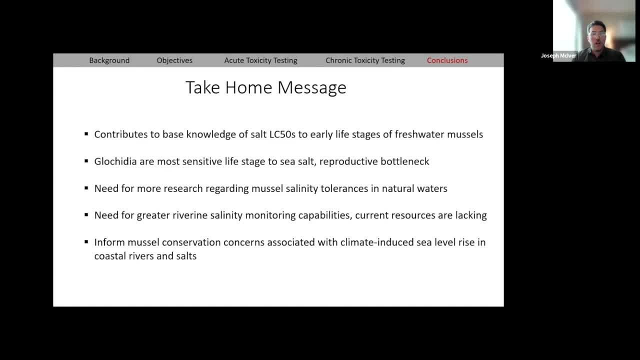 stages of freshwater mussels and previously unknown sea salt, LC50s. Glucidia, the most sensitive life stage to sea salt. So once again, that reproductive bottleneck. we want to, we want to protect the glucidia so that mussels continue to have stable populations. I think there needs. 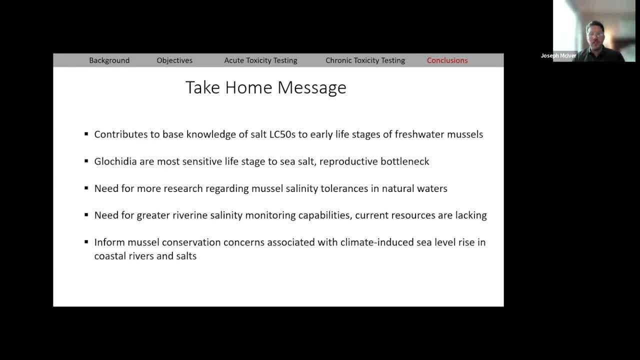 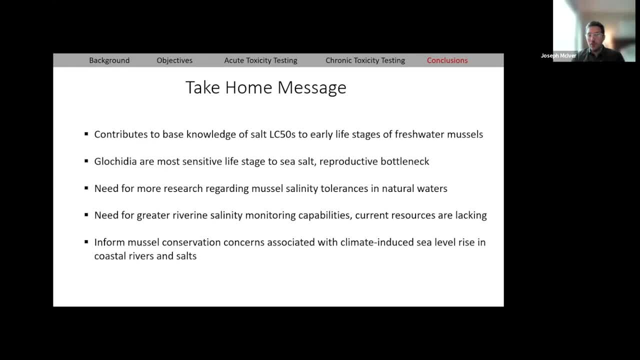 monitoring, salinity monitoring capabilities. um, in these lower portions of of rivers. Um, I had, uh, a little bit of difficulty finding um salinity data. Um, I kind of could find it for big like um, well-known rivers, but each river is different and salt's going to get into each 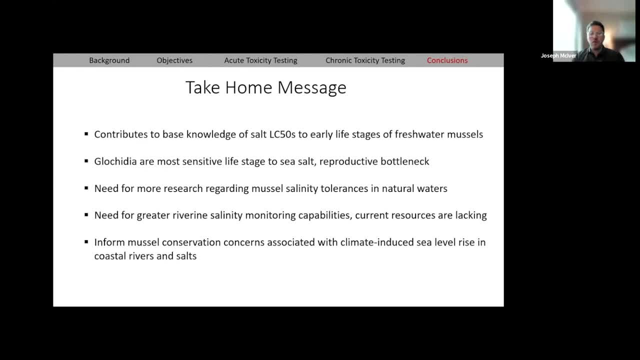 system differently and act a little differently, So it would be nice to have more widespread uh salinity monitoring capabilities And, lastly, um I think this can inform mussel conservation concerns associated with climate-induced sea level rise um in coastal. 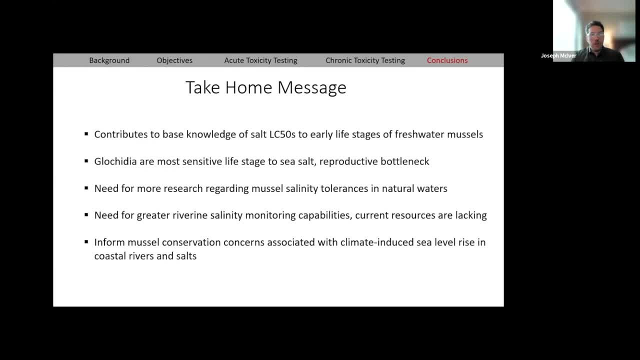 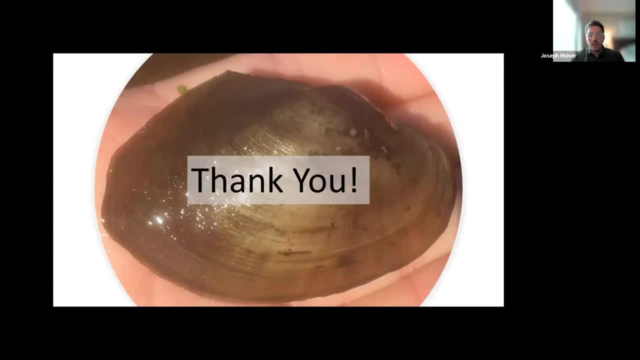 rivers and salts in general, So I think I went a little quicker than I wanted to. We're at 35 minutes, but I just wanted to thank um everyone here And if you have questions, I think, uh, we have time for that. Um, some, this is just a really cool um study with lots of elements. 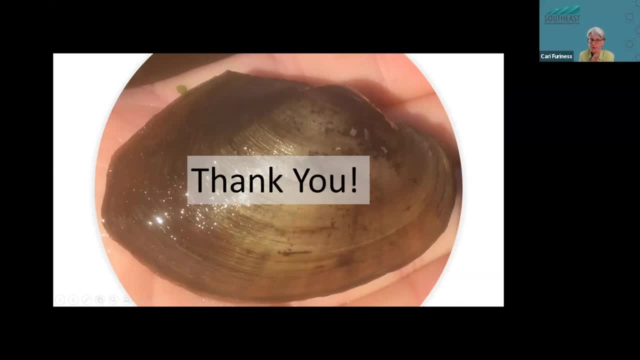 So um I'll open it up for questions and um Joseph is still sharing his screen. So if we need to go back to um, look at some of the data or um some of the results in in greater detail. 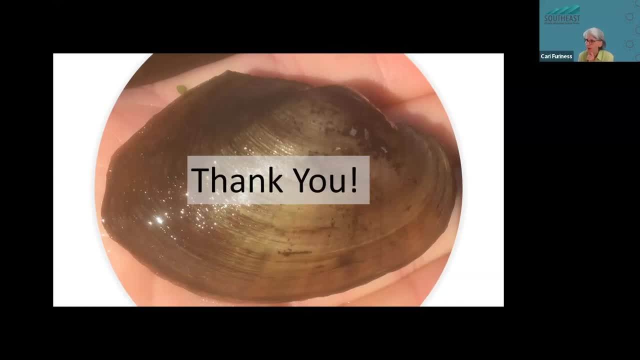 feel free to um ask for more clarification on that. All right, While people are thinking, I'm going to jump in with one. So um, um, Joseph, you mentioned the idea of some additional salinity monitoring needs Would. 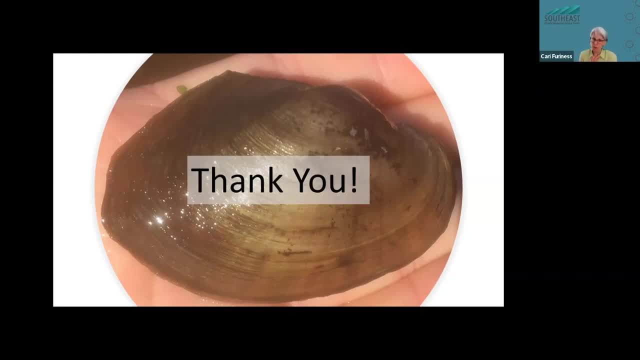 um. would would you be able to point to specific areas where that would be most relevant, based on um you know, your your knowledge of where some of these at-risk species in mussel species um exist, or where we we might like to have them exist, if they aren't currently? 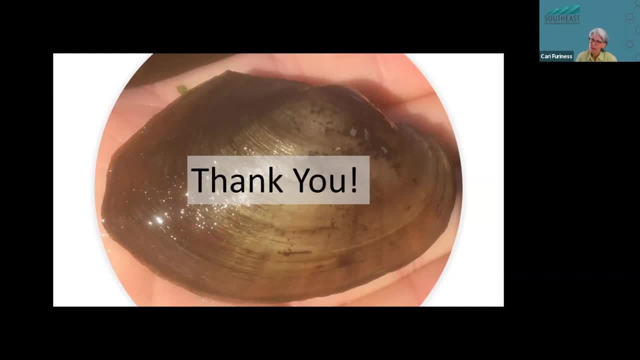 um, you know, viable populations there now. Um, I mean it'd be great to have them everywhere. I know that's not possible, but um, I mean we were working on that. Um, I mean we were working on that. Um, I mean we were working on that Um. 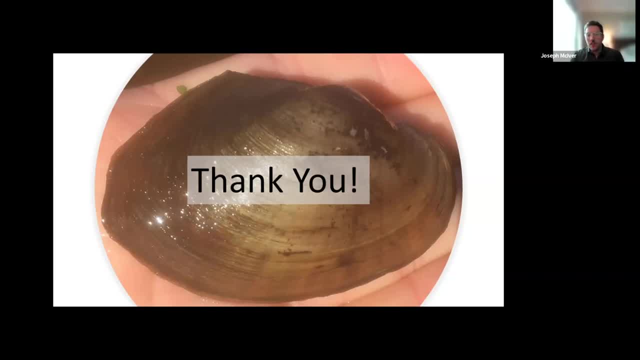 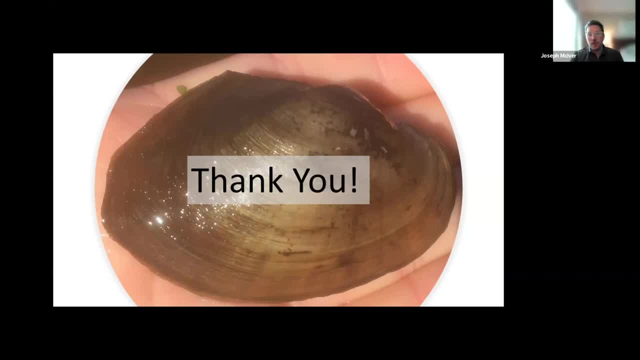 which is where those um okra were sampled from, And I found um. searching through the EPA STORET and kind of these water quality databases, I found um just a few, you know, spotty samples of salinity monitoring. 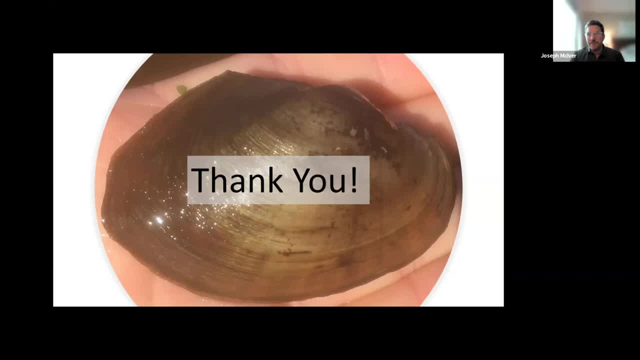 Um, so specifically, yeah, it would be nice to have it everywhere. Um, I didn't do it, but it worked. It worked really well. Um, and so I do, like this area, have much more than 70 species of olive leaf. forgive you, 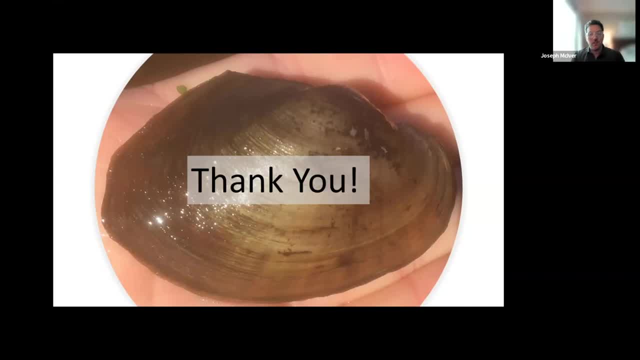 if I do like a huge population assessment on on where these mussels actually are. These were known locations provided by where the North Carolina Wildlife Resource Commission keeps, you know, keeps inventory essentially of where these mussels are, as well as the Virginia DWR. 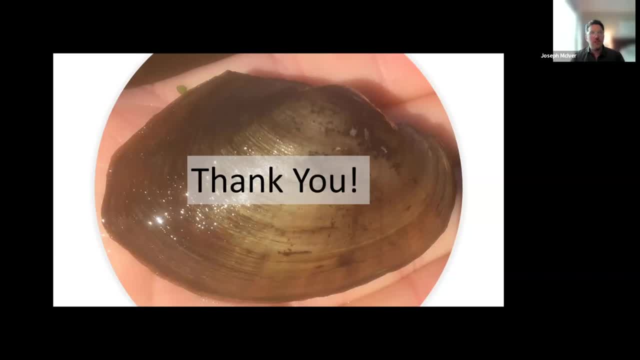 They collected the mussels. Um Yeah, I think those entities would have a great knowledge base of where you know where most of the muscles are, where they know that they are, and ones that could be used or focused on for some protection there. 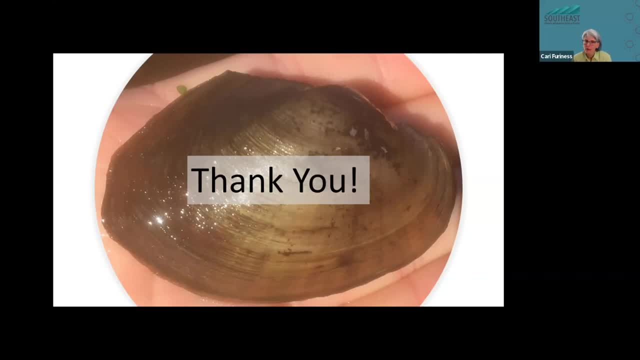 Great thanks. Other folks on the line have some questions. feel free to raise your hand or even just go ahead and unmute yourself If you have a question you'd like to ask, or put it in the chat if you prefer. I see in the chat says Maria Dunn she forwarded the NCDWR's ambient water quality monitoring for salinity. That's kind of some of the data I got into. 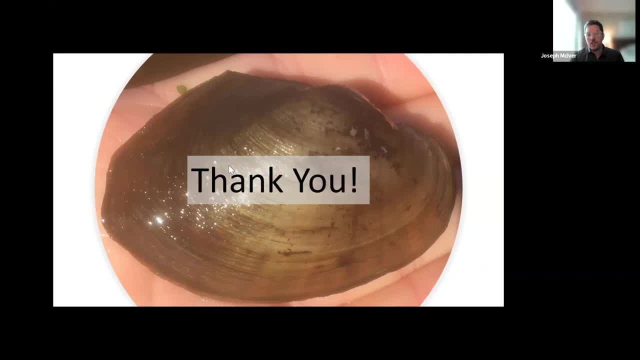 Which is where I found you know the Chowan at that collection site had experienced four parts per thousand of sea salt. It's just that they're so spotty like. it's like those were from 2008 or something like that. 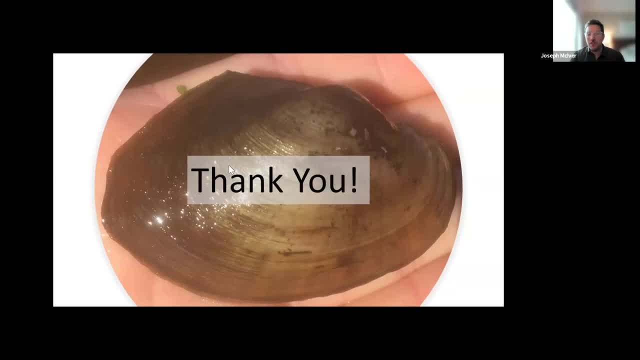 So you just don't get kind of a steady stream of data. Yeah, getting some good responses. I guess I'll just ask you, since we and I know you recently come through graduate program at NC State and are now moving into doing some of this. 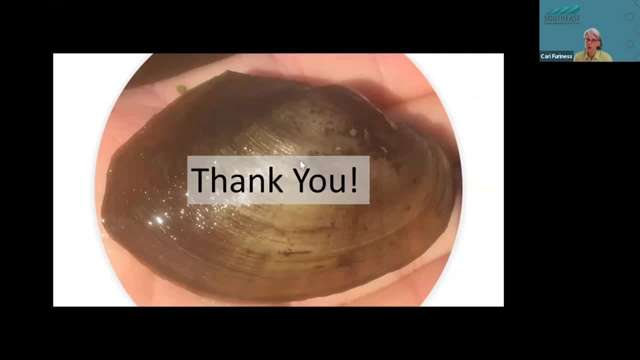 Some additional work professionally, If you were to suggest where are really some of- and you hit this a little bit on in some of your, so I don't want you to necessarily have to repeat yourself, but if you were knowing that there's researchers coming in behind you, if you were to. 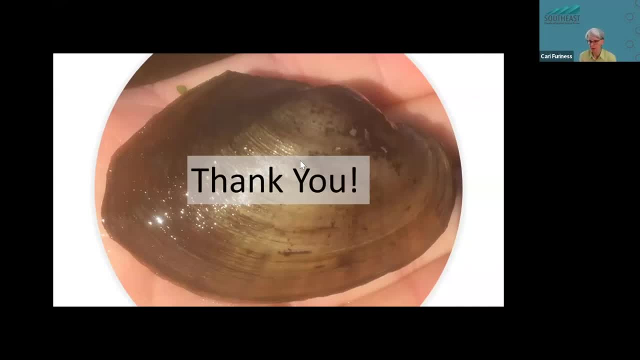 chat with a student to say here's where I think the next big- you know the next big research topic that would help inform some of these, you know, give additional information related to your research and, you know, help inform some of these decisions that may be needing to be made with increasing salinization and at-risk species, where would you suggest that students really put some effort? or other researchers, not necessarily students- 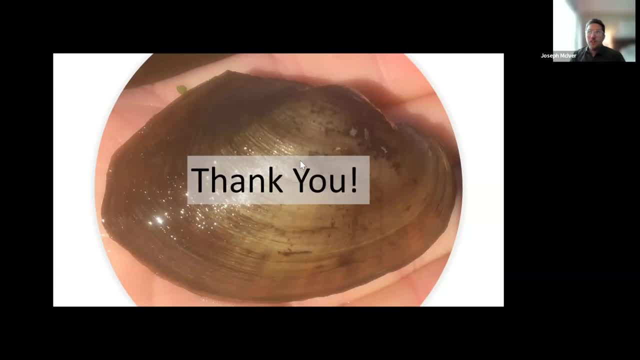 For me personally, the exposure to the mussels and salt in the natural water. I think that would be really really cool to look into Because EPA, when they set these water quality criteria- and they're typically done in the reconstituted water, which isn't as environmentally relevant- it's really good for comparative purposes. 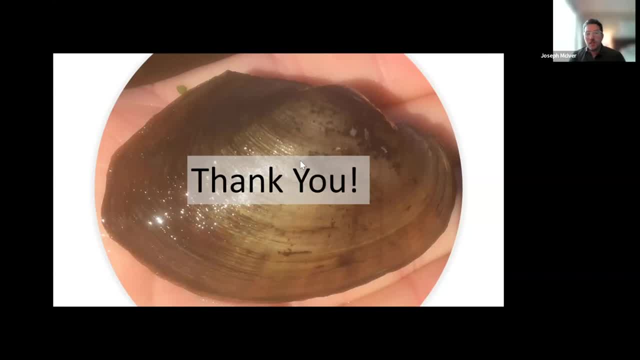 And it really might protect mussels more. but I think it would be nice to to see what they can stand in the natural water and maybe get get into more of what they actually can truly stand when they're exposed to it. in reality. It's just a lot of effort to do that. 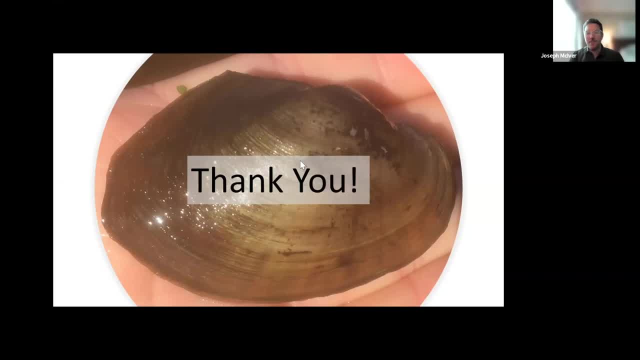 It's like you need a field lab, like right there. So it takes a lot, a lot more time and effort to kind of do that stuff, unless you're right at it. Right, Yeah, Yeah, that in situ. Okay, are there other folks that want to? 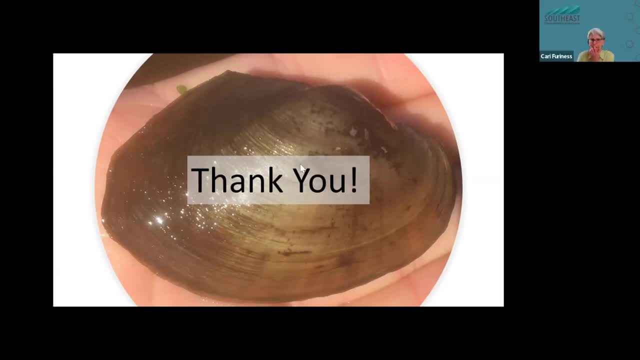 come in. Ryan had raised his hand earlier. Oh, I'm sorry, I'm not seeing that. Oh, here we go. And Charlotte, Sorry, I'm not, I was not looking at that box. Yeah, go ahead, Ryan. 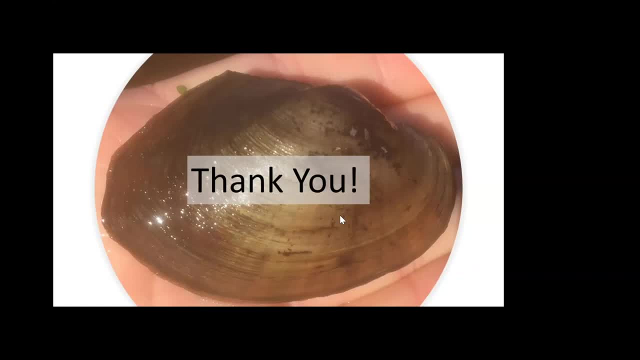 Thanks, Joseph, for the presentation. Very good job communicating that, You know. I see a couple of really interesting things from this research. First is, you know, just the testing of the different. you know how you think about the methods for exploring toxicity for some of these freshwater mussels. 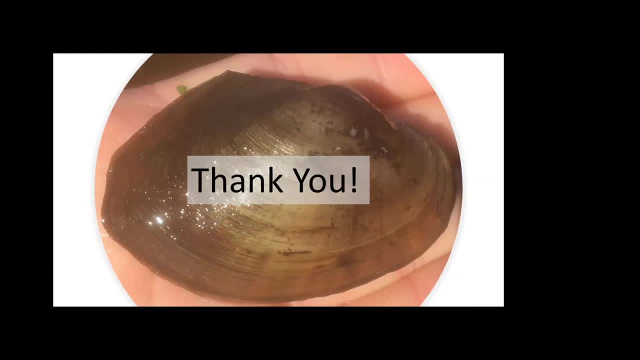 You know, testing the different methods, working that design out. That's really helpful And a lot of folks are going to be able to use that. The second that you know I have a question about is how. how representative are these mussels in terms of the broader set of freshwater mussels that are along all Atlantic rivers? 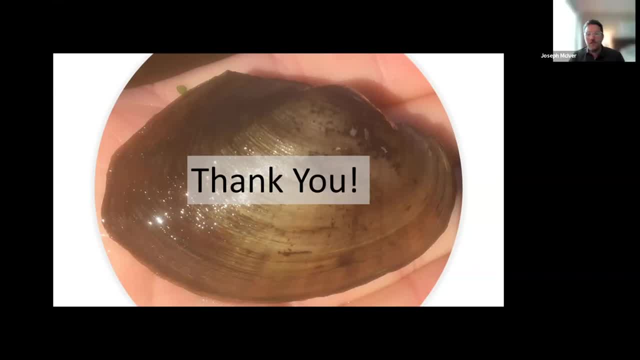 Are the conclusions for these specific species extendable to a lot of the others, Or is there or is there a lot of uniqueness among sort of you know species in terms of their biological functions that might make this really only relevant to these three species that you tested? 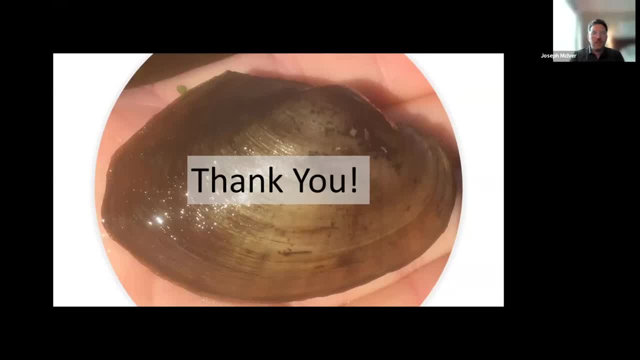 Right, That's a good question. I mean, it's obviously directly relevant to these three species. They have the same general functions- freshwater mussels, So it's relevant to all mussels, but you're never going to know who, exactly, what exact species of mussel it's. you know what exactly is going to happen to you know an elliptio that we didn't look at. 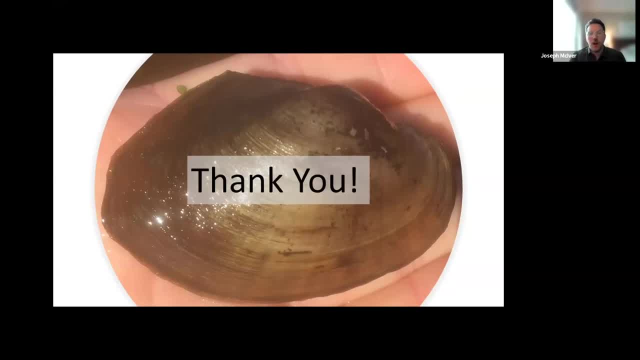 Elliptio mussels are everywhere and they seem to do really well. How are they going to react to sea salt under these same kind of samples? So I think this gives a good base amount of knowledge. But yeah, it would be. it would be great to continue looking at more species. 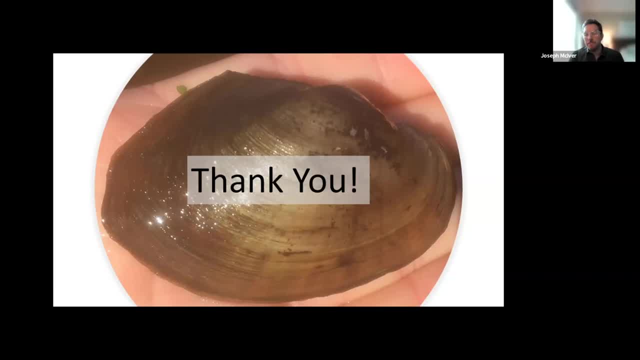 So, like for those, those, those Ooderbeke and Iplicata in the chronic test that were exposed to the salt in the reconstituted water that got wiped out, you know, would that happen within another species? Or would the Ooderbeke and Iplicata in a natural water? would they have persisted in that test? 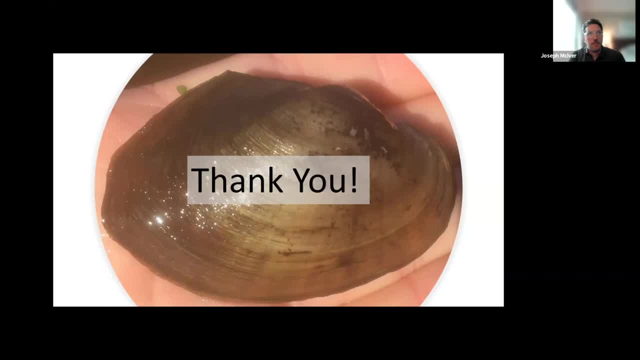 So generally, I think it's it is, it's it's informative generally, It would you know, always be awesome to know more about different species of mussels. Great thanks And sorry, I was not noticing the hands up earlier. Charlotte, you want to come in with your question? 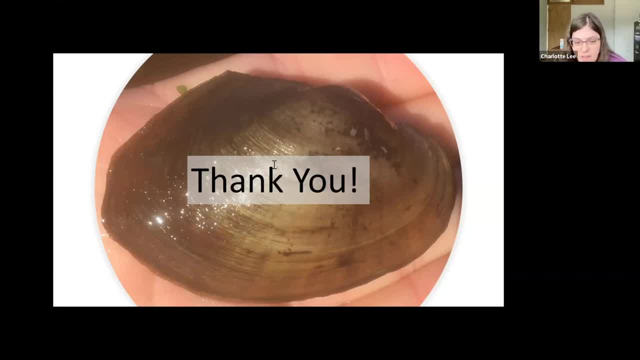 Sure. Thank you very much for the fascinating talk. I just started working with sea cask and I'm on a project related to sea cask. I just started working with sea cask and I'm on a project related to sea cask. 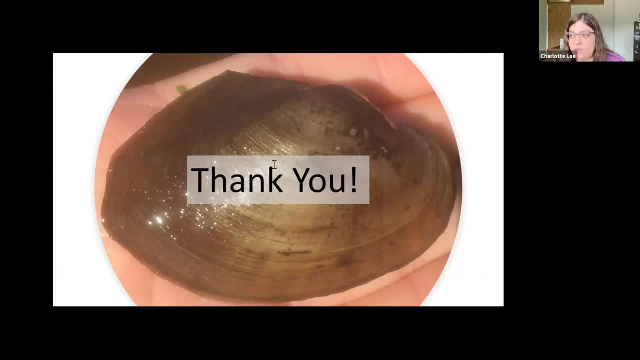 I just started working with sea cask, So my first question is related to how future changes in freshwater availability to coastal ecosystems is going to impact salinity and species. So I was curious in some of your background research when you were looking at these different tolerance ranges first, I was surprised to learn how focused everything. 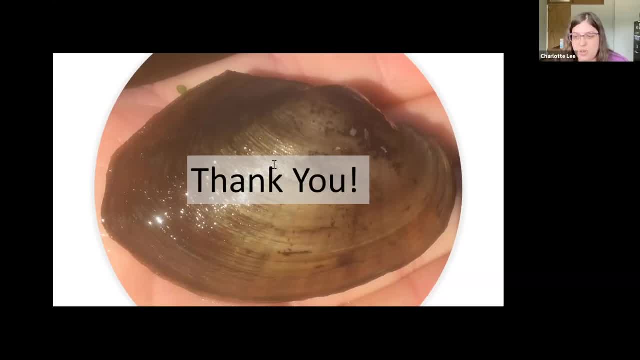 how focused previous studies were on just sodium chloride instead of natural sea salt. But my follow up is: is there a good resource or database related to these solidity tolerance literature, or is it kind of scattered everywhere? um, so i guess that was kind of my question is: how, how hard or easy is it to find some of this information? um, luckily, my advisor. 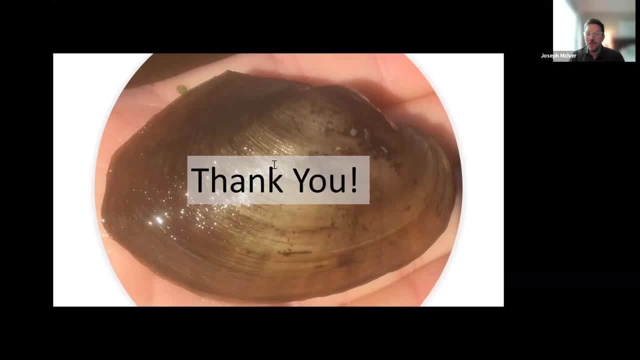 has been in the field a long time so he could pass a lot of these papers along to me. um, we're working on publishing the chapter one right now for the acute toxicity test, where i've compiled all of these salt ions into a massive salt table. um, so hopefully when that comes out, 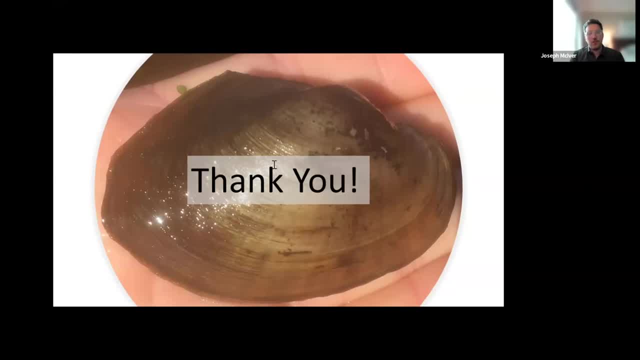 um that the paper we publish will be a good source where you could just um in the supplemental data, find all of that salt ion data, because it took a while to um get it all compiled, because it's quite a it's quite a bit of literature, but 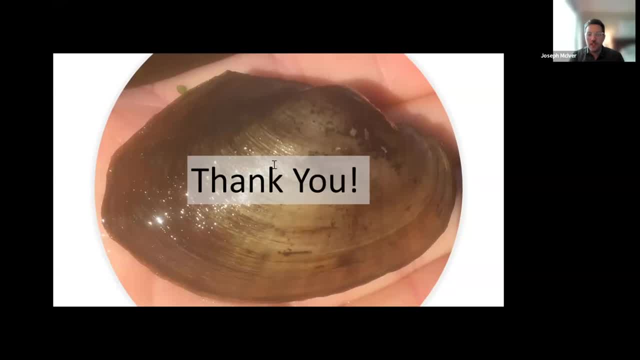 um, hopefully i can get it in in one place, at least for the time being. um, that sounds like it will be really cool and useful to the, to future researchers, and so, as that, as that comes out to publication, i definitely would enjoy to connect in and use that as a. 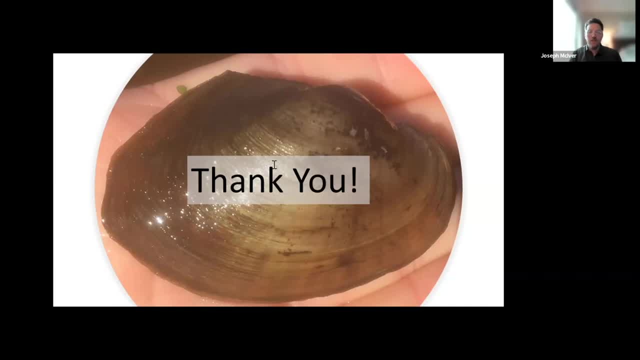 resource in some of my work. so thank you, yeah, thank you, yeah, great thanks. um other questions and i am looking at the participant box so i'll see if you raise your hand. um, okay, and thanks, britney, for putting um. you just, they just did produce a data release, that is. 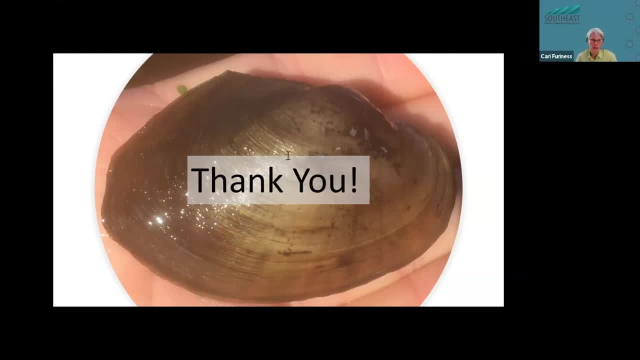 um now available from the project. so um, and we'll look forward to those publications coming out about it. um, okay, so not seeing other questions. well, we'll go ahead and um, just finish up and um, and then, if others come in, you can go ahead and chop them in the in the chat. 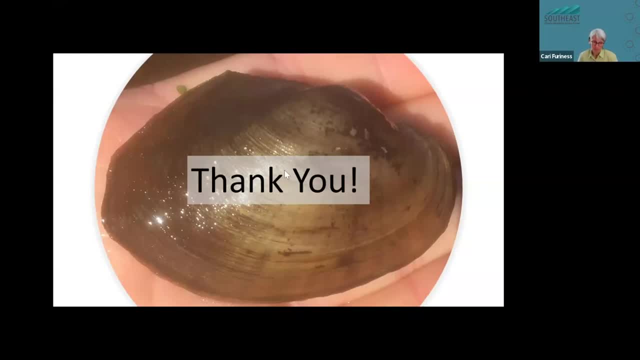 we'd like to go ahead And again say thanks again, Joseph, for this really really interesting presentation and really nice explanation of some of these results. Appreciate your being willing to share these with us and our users across the Southeast, And if you would like to stop your screen share, we'll let Kristen pop up with the last. 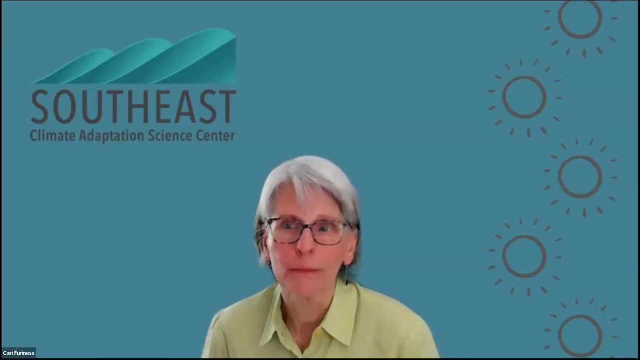 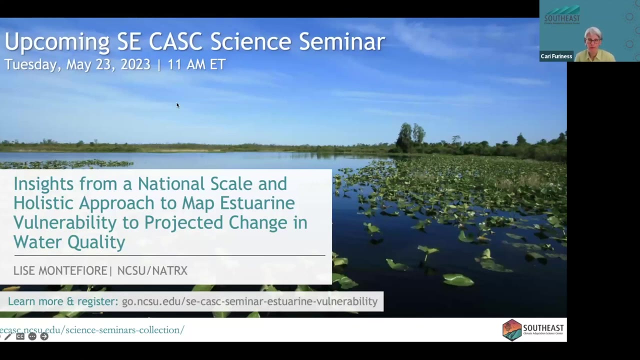 And I'd like to just wrap up by letting you know about our next CCASC science seminar, which is entitled Insights from a National Scale and Holistic Approach to Map Estuarine Vulnerability to Projected Change in Water Quality, And that's going to be presented by Lise Montefiore, who undertook this project. 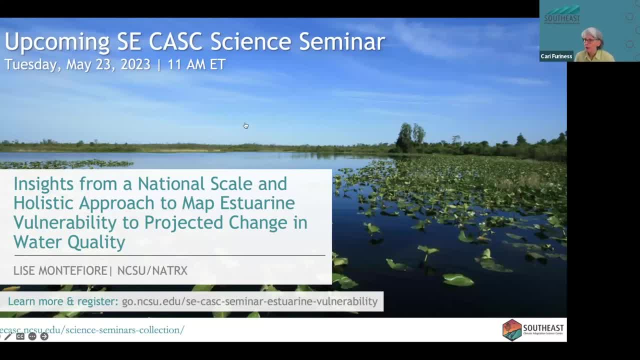 And was also one of our former Global Change Fellows. So Brittany has put in the link to register for that. We hope you'll join us for that seminar And wanted to also let you know that by registering for today's webinar we'll also be 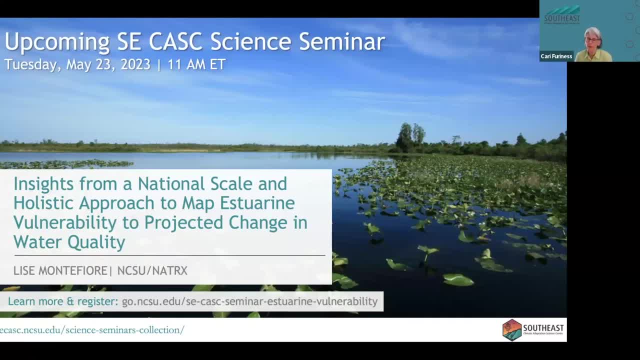 subscribed to our monthly newsletter, in case you aren't already, where you'll be able to learn about upcoming seminars and other events. Of course, you're welcome to unsubscribe at any time, But we hope you won't So. again, thanks to everybody for joining us today. 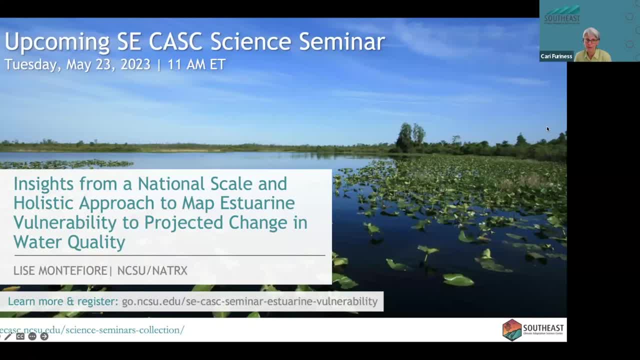 And thanks again, Joseph, For a really great presentation. So, seeing no more questions, we'll go ahead and finish and wish you a great rest of your day. Thanks everyone. Thank you for hosting, Thanks for having me, Thanks, Joseph.